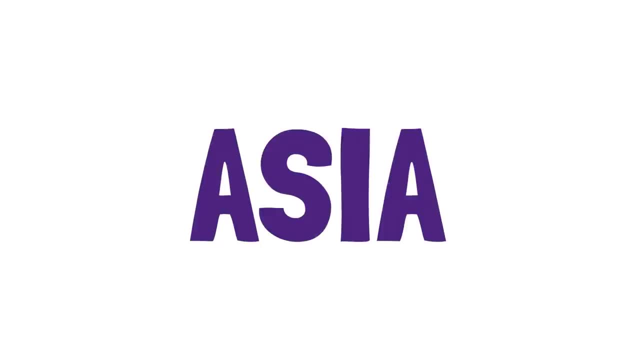 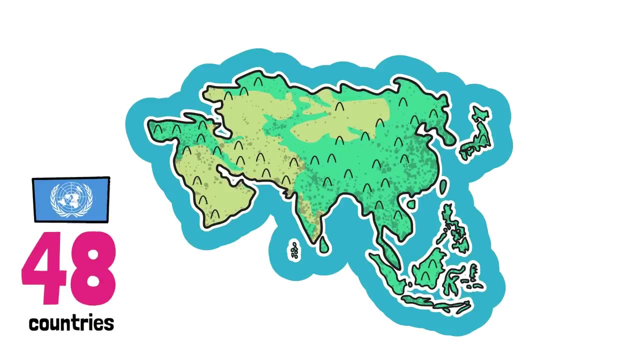 Asia. Asia has 48 countries, according to the United Nations, but for this video we're only counting 45, since I already covered Russia, Cyprus and Turkey's name in the European version of this video due to their partial belonging to that continent, and I'm including 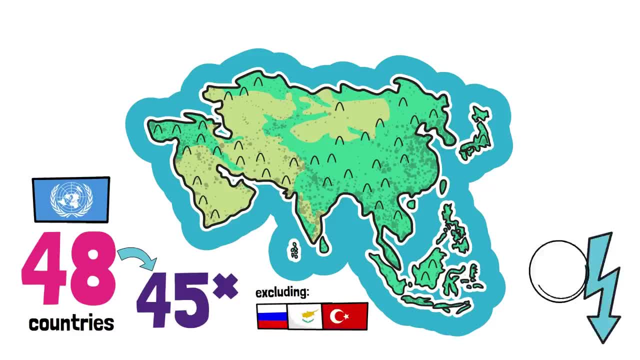 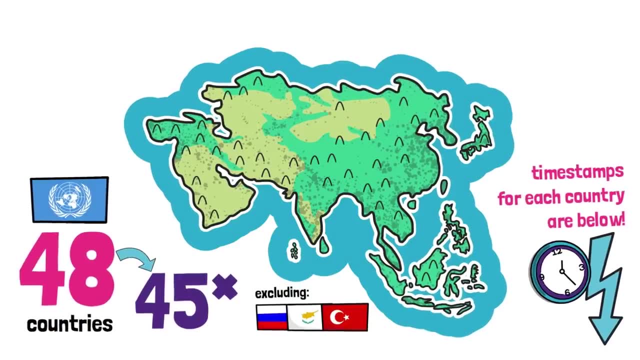 Timur in the one I make for Oceania. As usual, timestamps are in the description if you want to skip ahead to any country, since this is a somewhat long video and for each of these Asian countries I'm going to be looking at their name, origin, how it came to be, what it means and how it has. 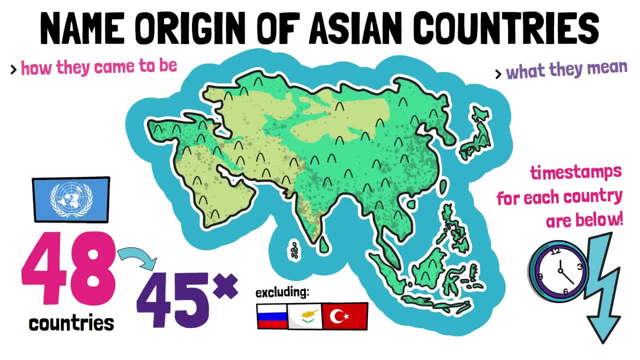 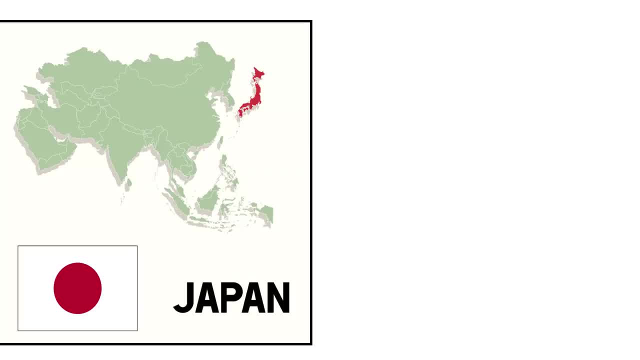 in some cases changed throughout history. For Europe we went west to east and for America we went alphabetically. so let's go east to west here, starting with the ones on the thumbnail. First, Japan. The name for Japan in Japanese is written using these kanji characters and pronounced: 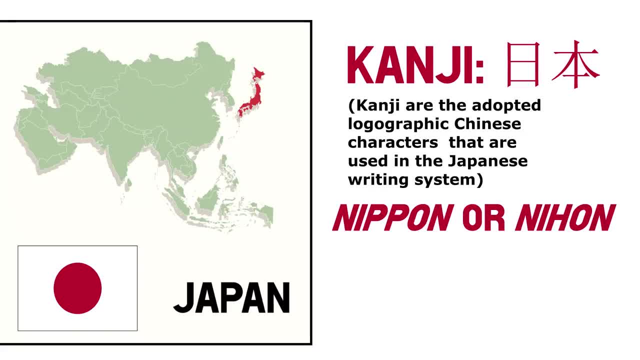 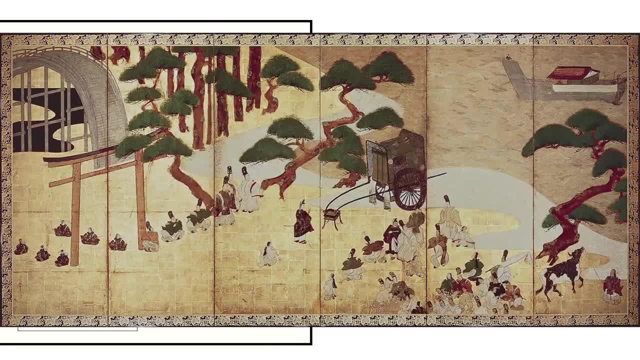 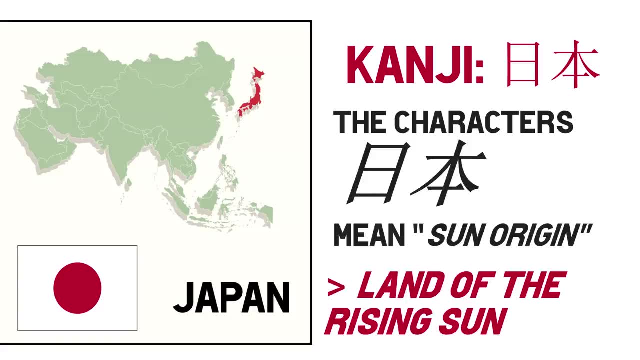 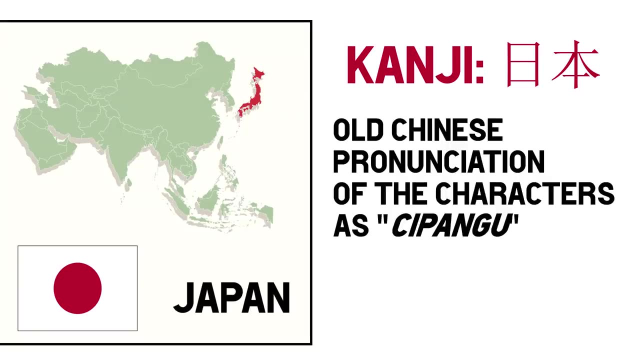 and in Japan by Yamato. The characters mean sun origin and are therefore the source of the popular western meaning attributed to Japan: land of the rising sun. The western name Japan itself comes from either the old Chinese pronunciation of the characters as Sipangu or from the old 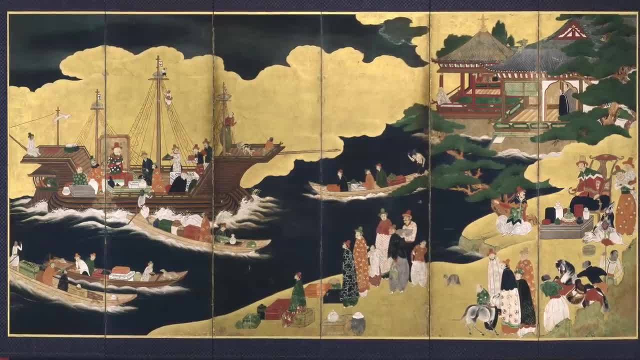 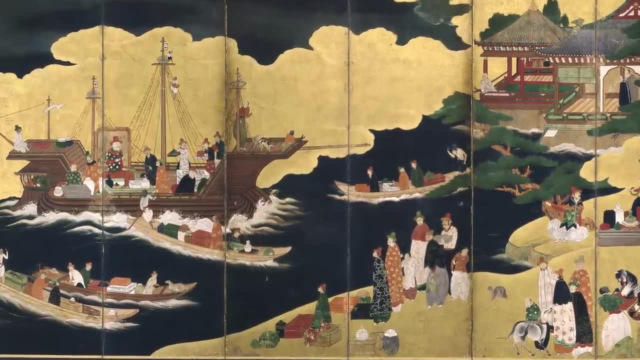 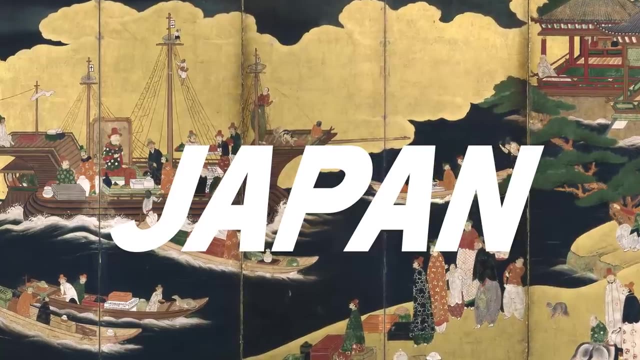 Malay name for the country, Japang, which the Portuguese brought back to Europe after their exploration of Southeast Asia. The English then translated a Portuguese letter referring to these lands, translating it to Chiapan, which eventually transformed into the current Japan. Then on to another archipelago, the Philippines. The islands were named by Spanish explorer. 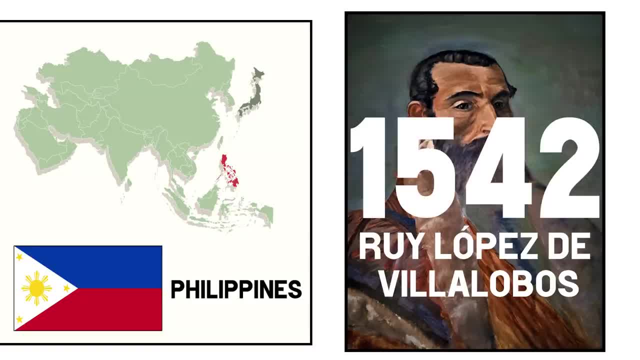 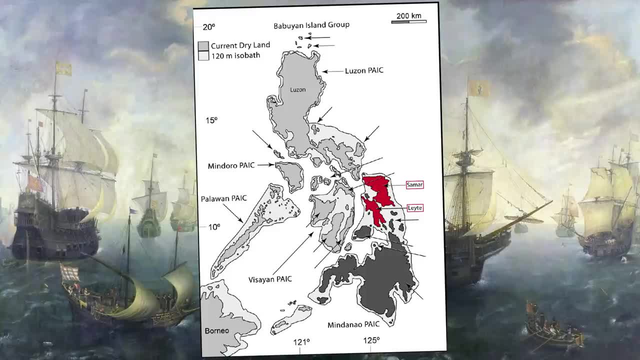 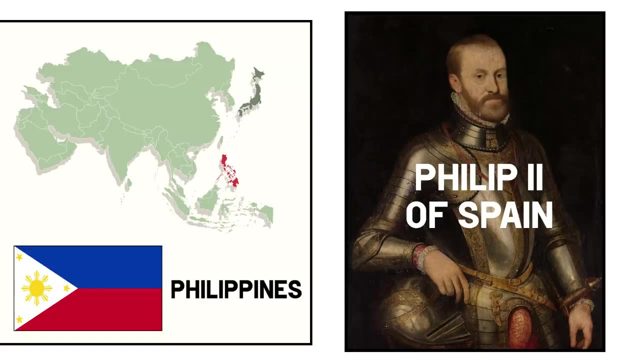 Rui López de Villalobos In 1542, he encountered a number of islands, naming specifically the islands of Leite and Samar as Filipinas, after the then Spanish prince, soon to be king Philip II. Eventually, this name was applied to all of the islands in the archipelago, which were: 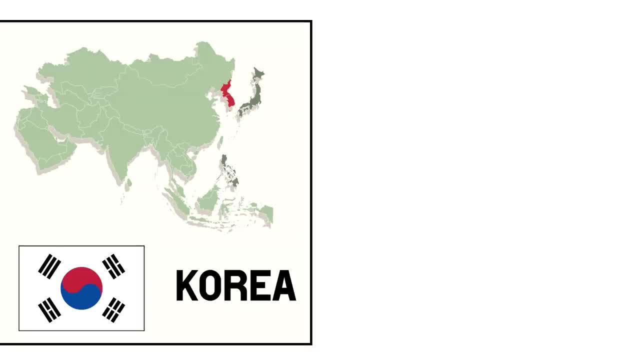 at the time the Philippines. The Philippines were named after the Spanish king, Rui López de Villalobos, under Spanish possession. Moving to the Koreas, the only difference are the north and south elements, so we can cover the name origin of the two together. The name Korea derives from the name. 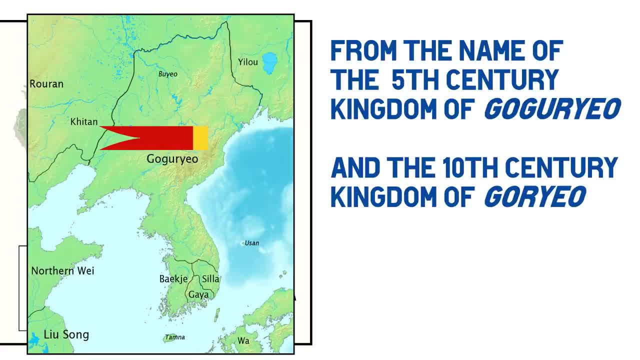 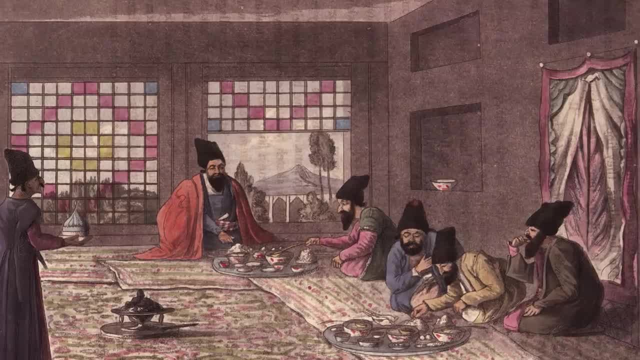 of the ancient 5th century kingdom of Goguryeo and then the 10th century kingdom of Goryeo. It seems that around these times, visiting merchants from Persia adopted the name to Korea, but it seems to be a coincidence that this Persian translation is the same as the current English. 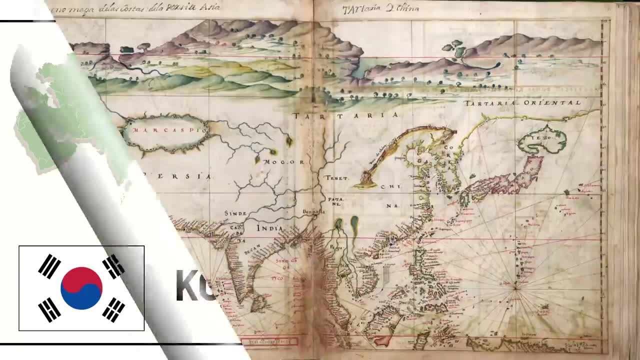 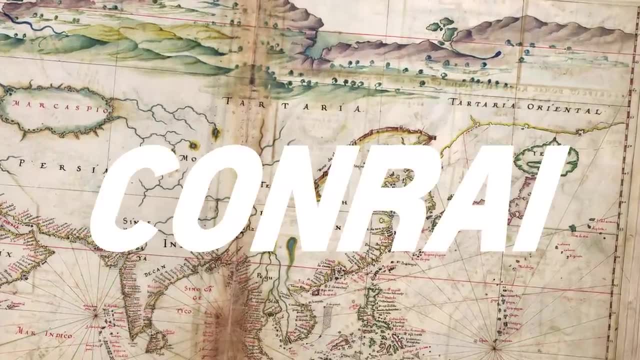 one, because the modern name of Korea apparently comes from the Persian name, which is the Portuguese maps from 1568, made by explorer João Vaz Dourado, who wrote the name of the peninsula as Conchay with another explorer in 1630, then changing the name to Korea. Maybe this? 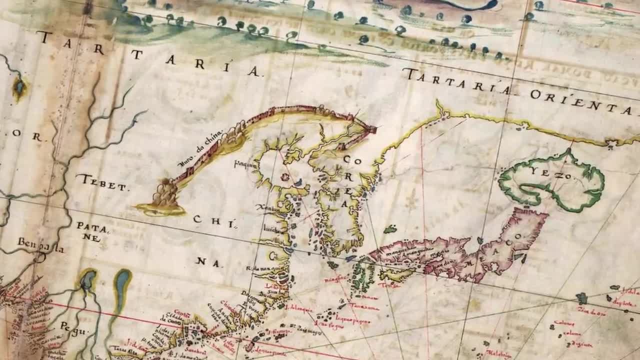 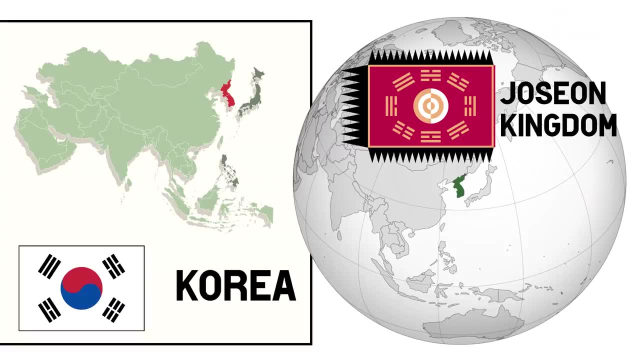 came from the Persian translation, maybe it came from the native way of describing it, I'm not sure. Eventually, the kingdom of Goryeo was replaced by the Joseon kingdom and then Dayan-Jeguk, which was the empire of Korea. Essentially, it seems that the Koreans themselves have always 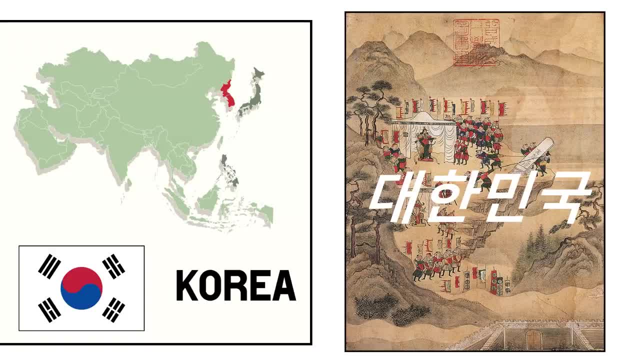 referred to their country in their own way and, like the Koreans themselves, they have always referred to their country in their own way and, like Japan, Korea was just the adaptation that Westerners created to refer to it. Going south to Taiwan, the island where Taiwan is. 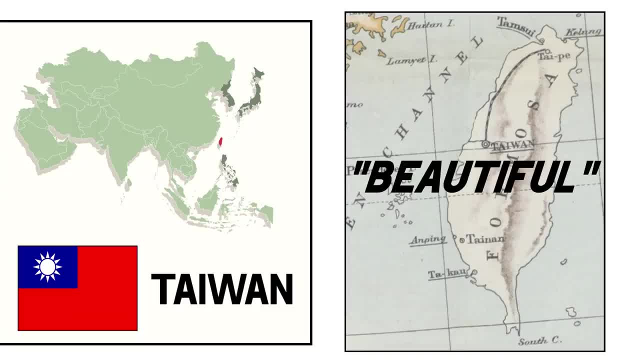 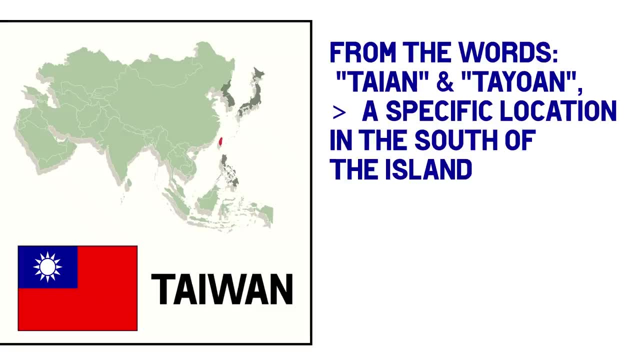 located has had several names throughout history: Formosa meaning beautiful, a name chosen by the Portuguese once again when they sighted the island in 1542,, while Taiwan itself seems to come from the words Tayan and Taiwan, the local terms used to refer to a specific location in the south of. 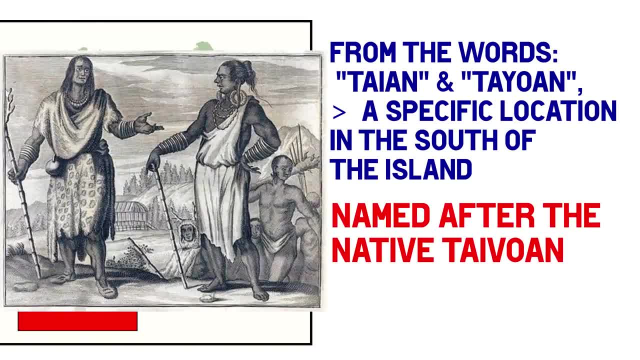 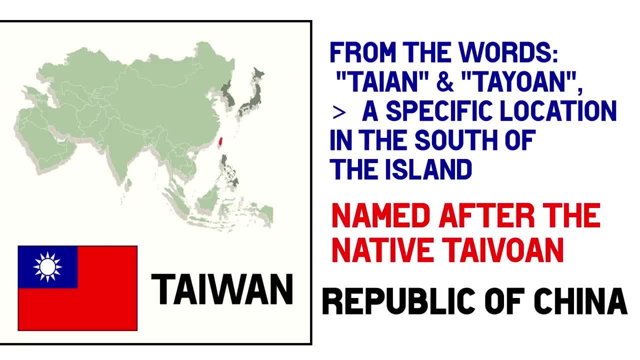 the island. This area is likely to have been named after the Taiwan people who are native to the land. Its official name is Republic of China, differentiating itself from the People's Republic of China, since the two sides opposed each other in the country's internal conflict. 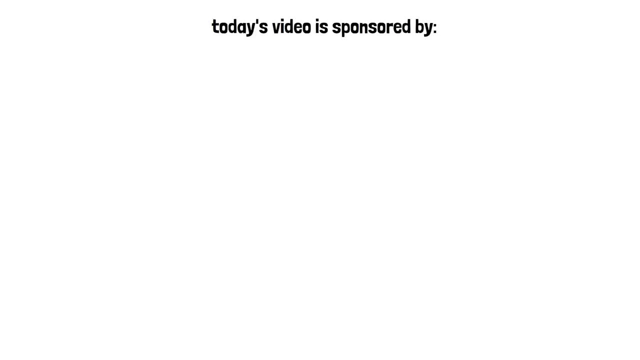 of the 20th century. Before we go on with the video, a quick message from our sponsor and friend of the channel, Blinkist Guys. I love Blinkist. I'm not even saying it because of the sponsorship. I actually pay for a Blinkist account ever since they sponsored the first video here on 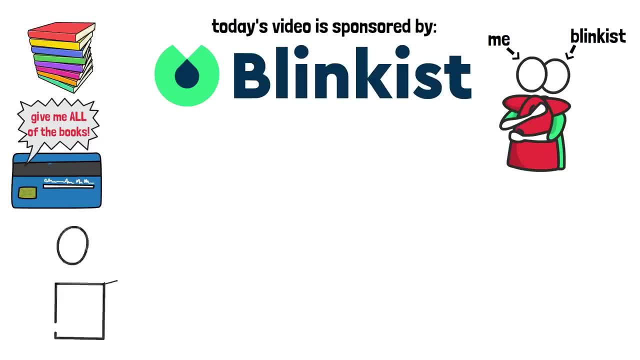 the channel. I got to know them and their service is just incredible. Everybody wants to read, but we either don't have the time to read it, or we don't have the time to read it, We don't have enough time, or our attention spans are so small because of all the fast media we 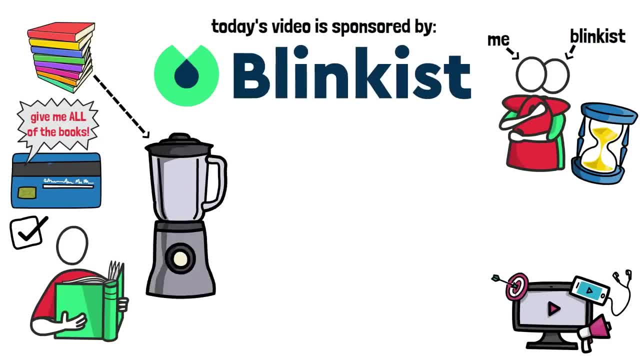 consume, so we end up not doing it. Blinkist solves that problem. They take thousands of books and condense them into around 15 minute listening or reading sessions with all of the key points you need to know. They only do it for non-fiction books, so you can still spend all. 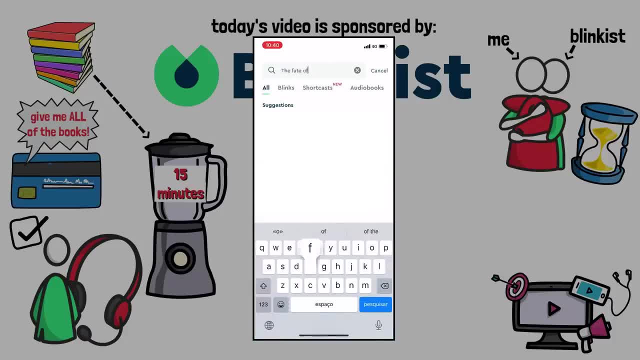 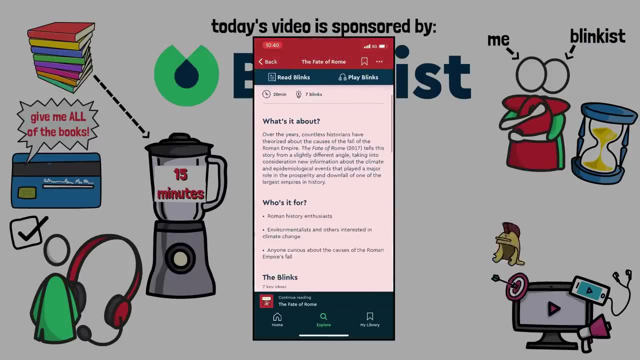 those hours reading chapter 14 of the Silmarillion, all of the mountain descriptions, Anyway. I even use it to find ideas for videos sometimes, or just to listen to topics I like, such as the history, like this great one about the fate of the Roman Empire, The first 100 people to go to. 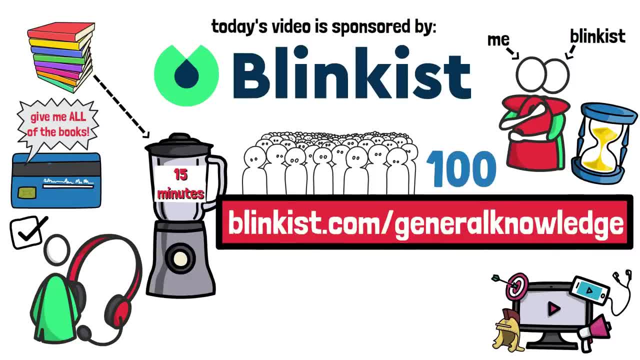 Blinkistcom slash general knowledge. get unlimited access for one week to try it out for free, and you'll also get 25% off if you want to continue with the full membership after that. Thank you to them for sponsoring the video. now let's get back to the countries And moving precisely to 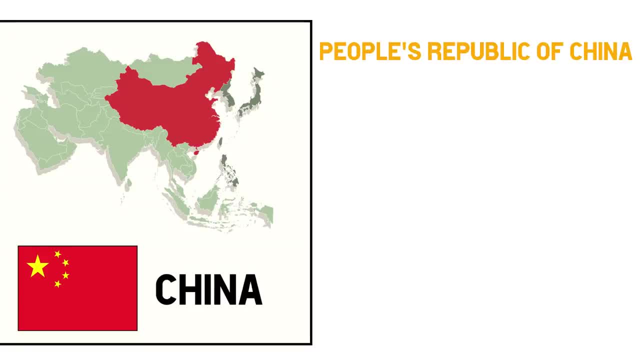 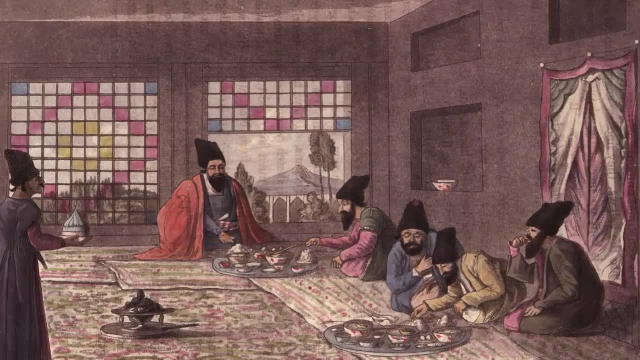 China itself or the People's Republic of China, rather similarly to Korea. The adaptation of the name that eventually led to the western version of it comes from the name Blinkist From Persia. The word China has been used since the 16th century, but it doesn't come from the. Chinese themselves. In 1516, Portuguese explorer Duarte Barbosa published a journal, and in it he referred to the land of China as such, but he didn't make up the name. It was derived from the Persian word Chin, which in turn came from the ancient Sanskrit dialect's word Sina, dating back. 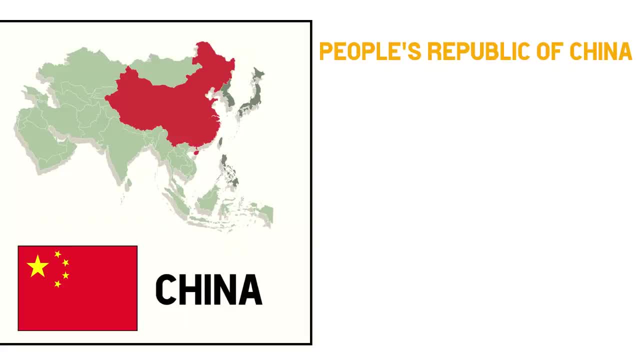 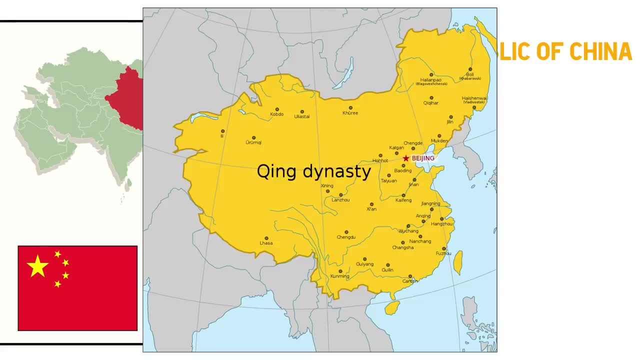 all the way to the 5th or even the 2nd century. Most people claim Sina itself was a way of referring to the land under the rule of the Qing dynasty. The word China is a word that is used to describe the Qing dynasty. This is unconfirmed, but a likely origin. The Chinese themselves refer. 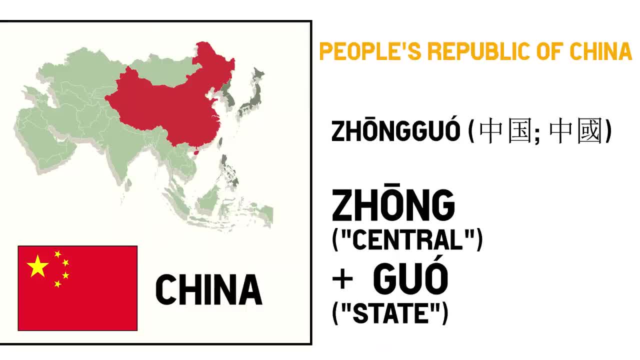 to their country as Zhonggu, from Zhong, which means central, and Gu, which means state, Although it could also be translated as Middle Kingdom, and it likely initially referred to the western and then eastern Zhou dynasties and their control over vast parts of China. 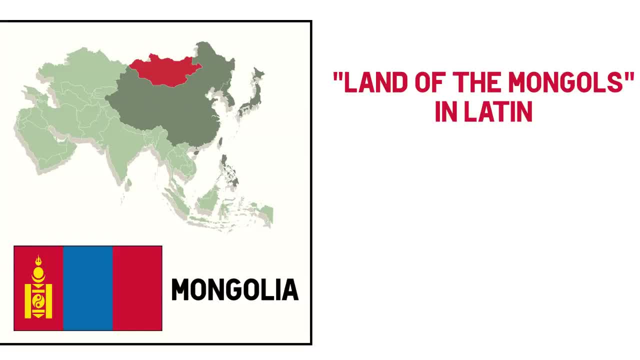 Going north to Mongolia. Mongolia literally means land of the Mongols in Latin, and Mongols is the native word the locals use to describe themselves, but its origin is uncertain. There are various options, like it coming from the native name of a mountain or river, or from the Mongolian. 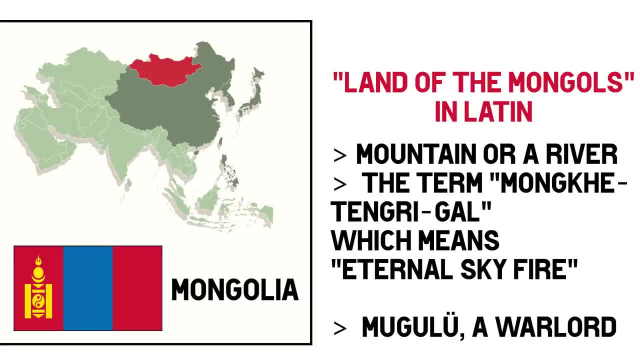 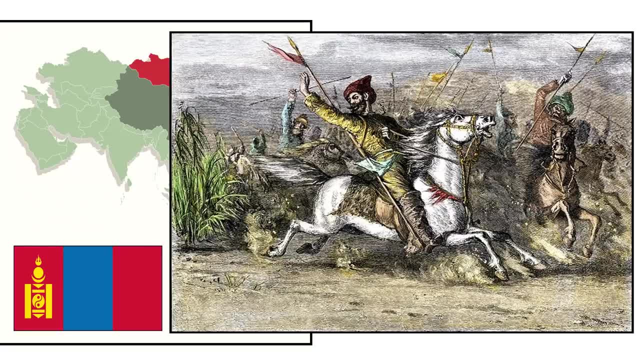 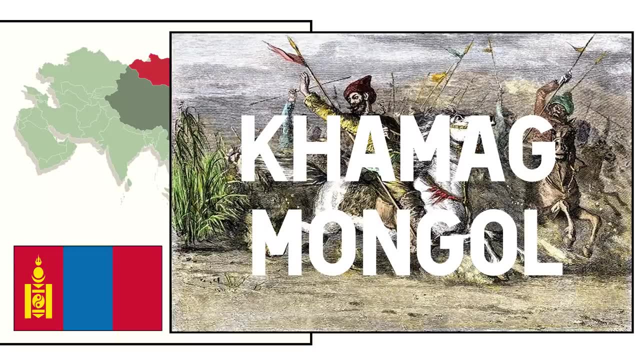 term Mongke Tengrigal, which means eternal skyfire. a pretty cool name, if I'm being honest, But the most likely origin is that it comes from the name of a specific tribe named by the Chinese as Mungu or Mungku, which then became known as the Kamag Mongol, a leading tribe which eventually 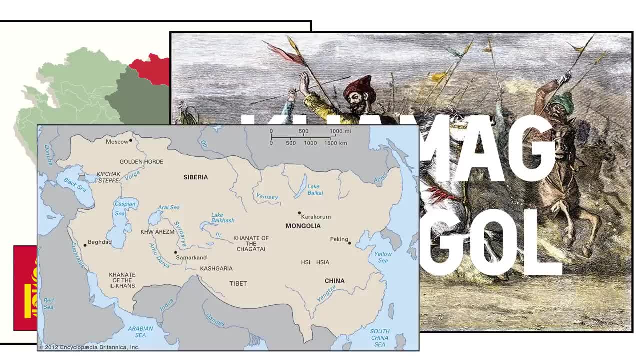 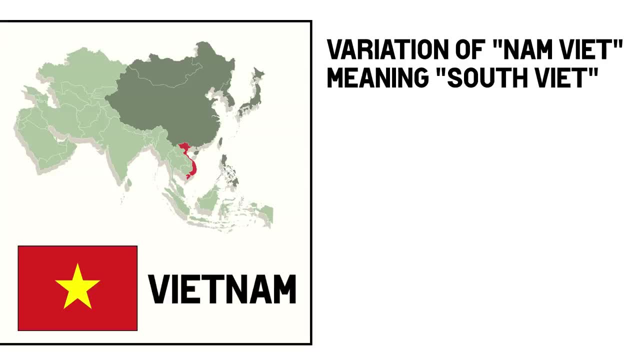 led to the creation of the Mongol Empire, causing all of the Mongol people to be known under this name, All the way south again to Vietnam, which is a very common name for the Mongolian people. This is the origin of Nam Viet, literally meaning South Viet, and this name can be traced all the way. 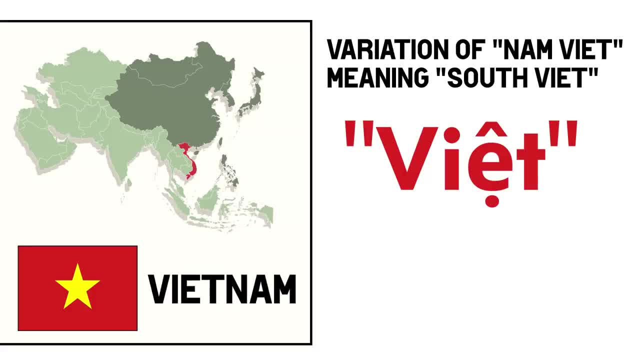 back to the 2nd century. The term Viet was apparently first used by the Chinese and referred to a people or a chieftain in the area Yue, as they pronounced. it was apparently even used by them to refer to non-Chinese people in southern China. Anam was apparently a common name for the 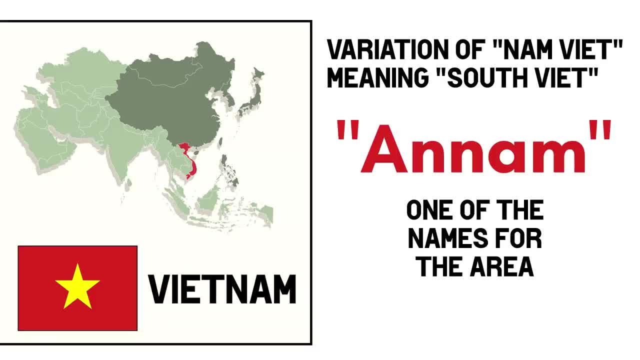 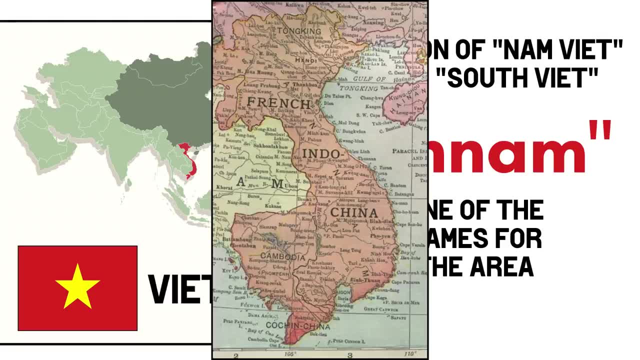 area as well, But the region has had many names throughout history: Van Lang Nam, Viet Aninam, Dai, Viet Dainam, and then being a part of an area which has been known during European colonialism as Indochina or Xiuqin China, until becoming 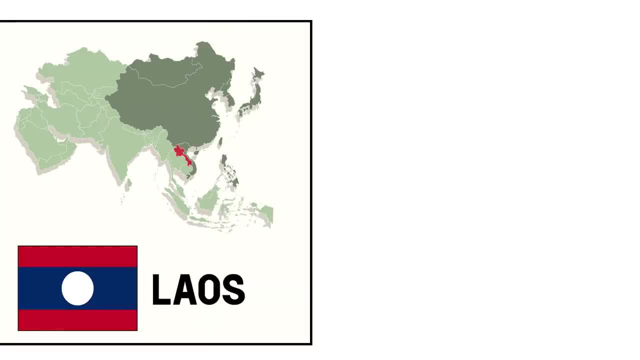 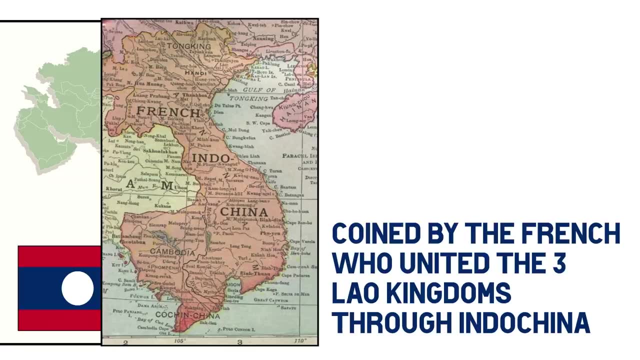 known as Vietnam. again Close by is Laos. The term Laos was coined by the French, who united the three Lao kingdoms through their colony of French Indochina in 1893, and named the country after the most common native group, the Lao people. The origin of the name Lao itself is apparently unknown. 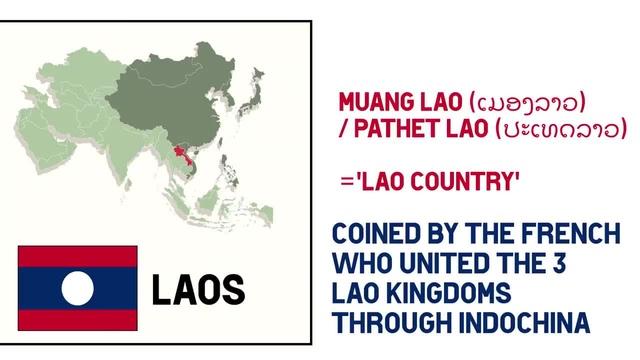 and simply dates back to the name of an ancient tribe from which these people originated. In the Lao language, the country's name is Muang Lao or Patet Lao, both of which literally mean Lao country, Still in the area Cambodia. The English Cambodia is an adaptation of the French. 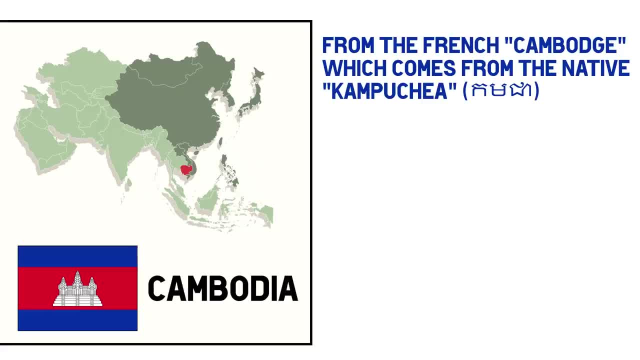 Cambodge, which in turn is the French translation of Kambucha in the native Khmer language. Its origin comes from the ancient Sanskrit language and the joining of two words: Kambuja, which refers to the foundation myths of the first ancient Khmer kingdom, and Deza, which means 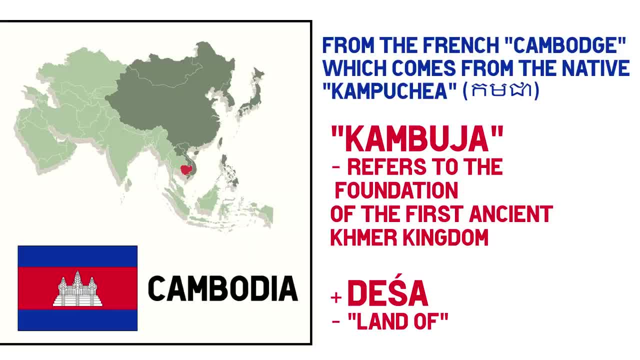 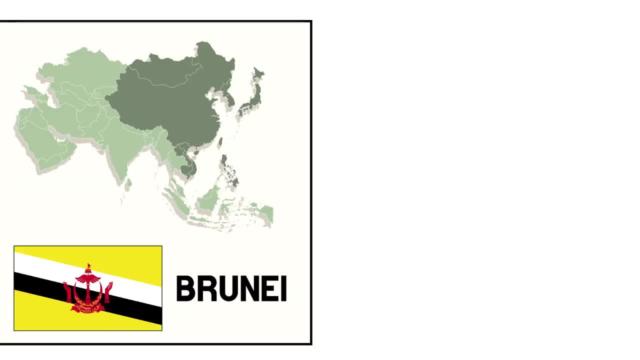 land of or country, So essentially the name would be Land of the Khmer, I think. Continuing south to Brunei, This one has a crazy origin. if we are to believe the story, Brunei was founded by Awang Alak Betatar, It is said, the soon-to-be first Sultan of. 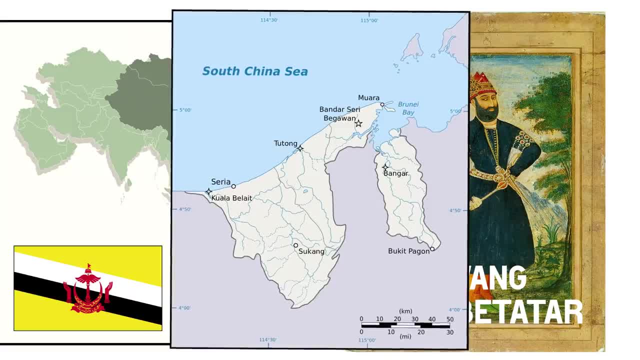 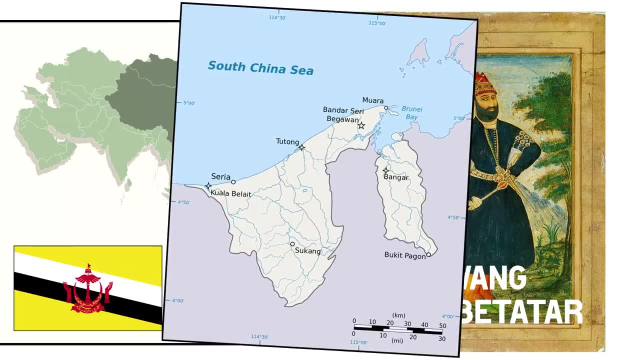 Brunei was searching for a location in which he should establish the center of his domain, And when he arrived to the estuary of what is now the Brunei River, he, according to legend, exclaimed Baruna, which loosely translates as that's it from which the name Brunei would. 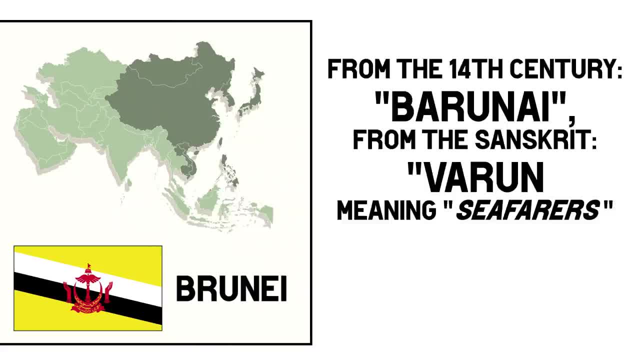 eventually derive. But a more likely explanation is that it comes from the 14th century word for the area, Barunai, which would come from the Sanskrit Varun, meaning seafarers, with the word Borneo, the name of the entire island having the same origin. 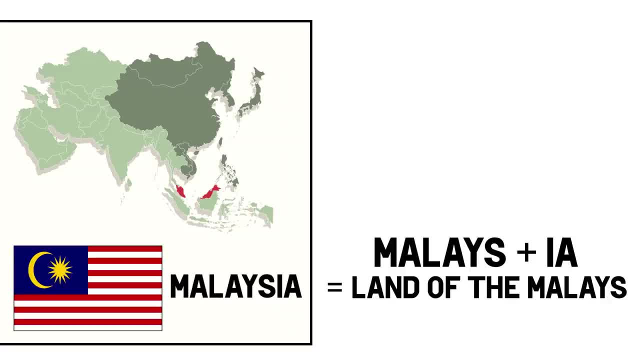 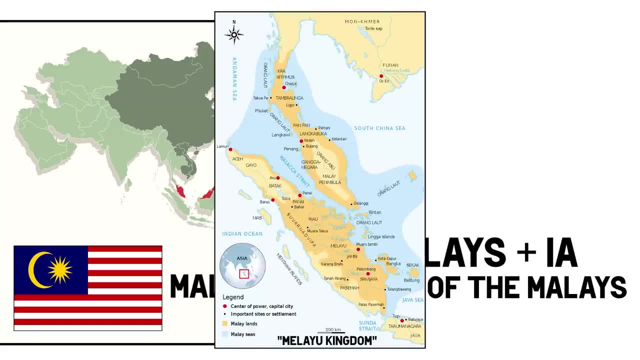 And around it Malaysia, A combination of the words Malays and the suffix ia. it can be translated as land of the Malays. An ancient kingdom existed in part of continental Malaysia, called Melayu Kingdom, around the 6th-7th century, and it seems that is the first origin of Melayu. 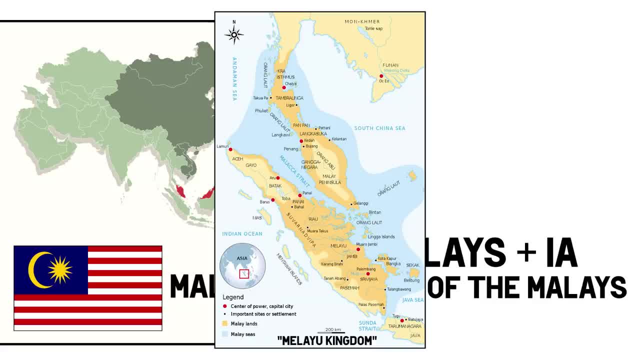 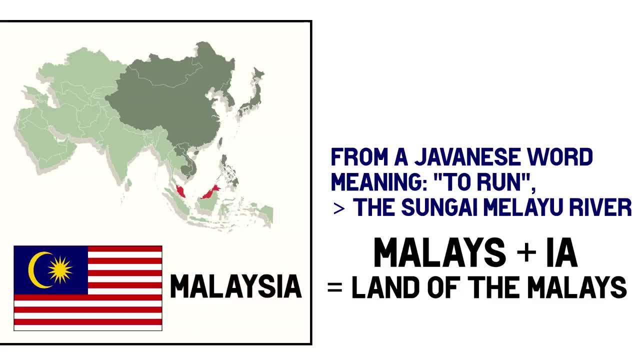 But the origin of Melayu itself is uncertain. The main suggestion is that it derives from a Javanese word meaning to run from the name of the Sungai Meliau River, But we can't really be sure, especially because it seems to have always had this name In the 2nd century. 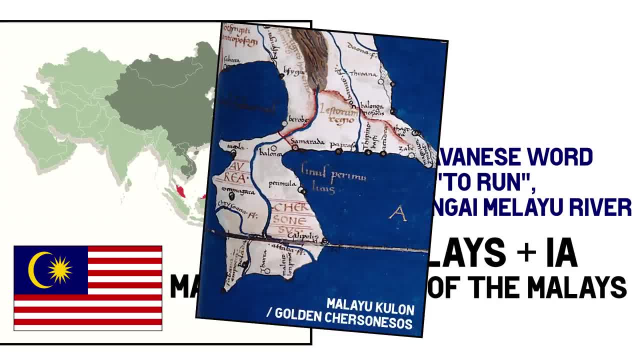 Ptolemy's Geographia used the name Malayu Kulon to roughly describe the area That Melayu Kingdom also reached into the next country, Indonesia, joining two Greek words, Indos and Nesos, and meaning Indian islands. In 1850, George Windsor, an Englishman, was born in Melayu, and he was born in Melayu. In 1850,, George Windsor, an Englishman, was born in Melayu, and he was born in Melayu. In 1850,, George Windsor, an Englishman, was born in. 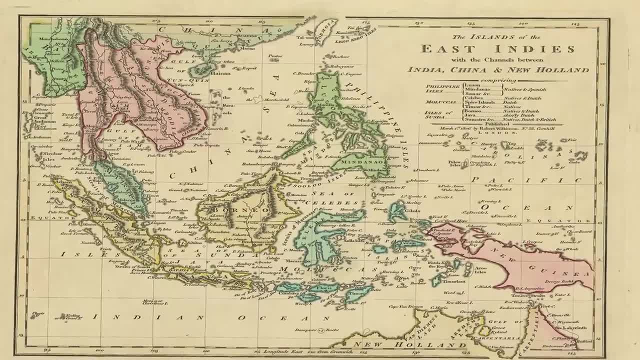 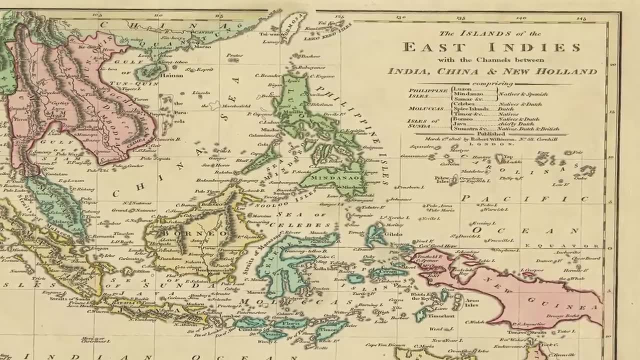 Melayu. In 1850,, George Windsor, an English researcher, proposed the term Indonesians and Melayunesians for the inhabitants of the Indian or Malay archipelago. It was also briefly known as the Dutch East Indies when it was ruled by the Netherlands during colonial times. 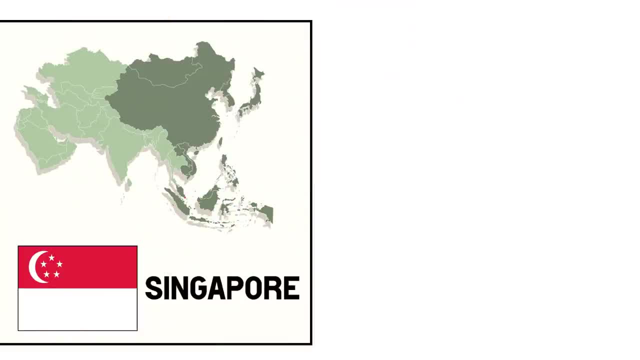 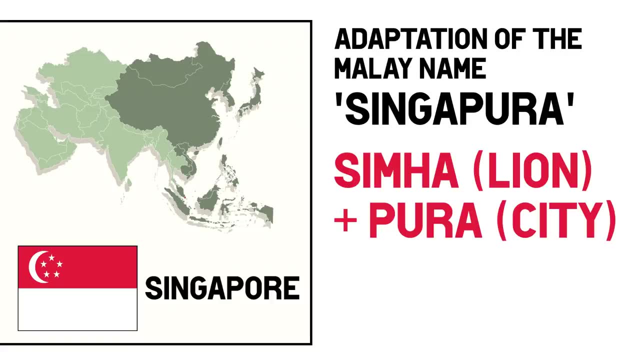 Back to the mainland, the small city-state of Singapore. Singapore is an English adaptation of the Malay name Singapura, which was in turn derived from a Sanskrit word meaning lion city. Simha means lion and Pura means city or fortress. 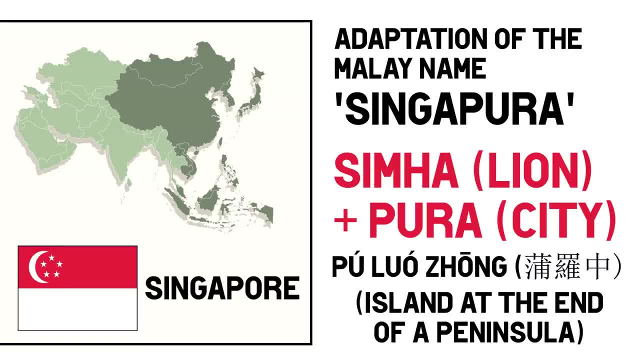 An ancient Chinese account from the 3rd century referred to it as Pu Luo Zong, which would translate to island at the end of the peninsula, an accurate description for its location Under Japanese occupation. Sionan meaning light of the south. then returning to Singapore, 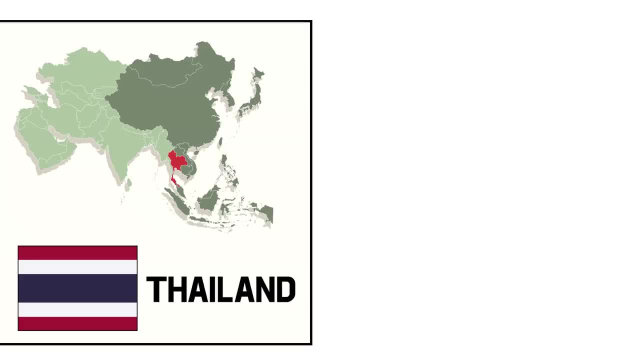 when the occupation came to an end. Further north is Thailand. The country has always been called Muang Thai by its citizens, but for outsiders it used to be known as Siam, then changing it to Thailand. So we need to take a look at the origin of both of these. 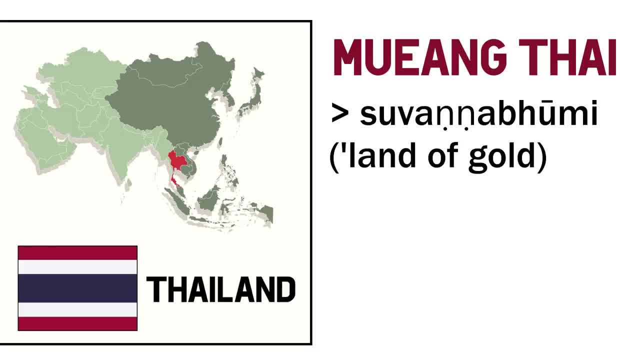 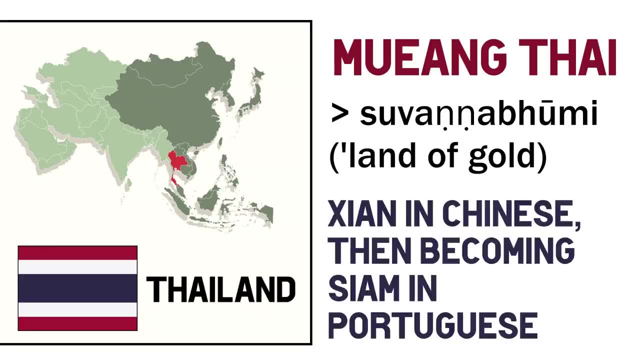 The word Siam may have originated from Suvarnabhumi, meaning land of gold in the Pali language. Another theory is that the name derives from the Chinese, who called the region Xi'an, which the Portuguese converted into Siam. According to a French scholar, Thailand means 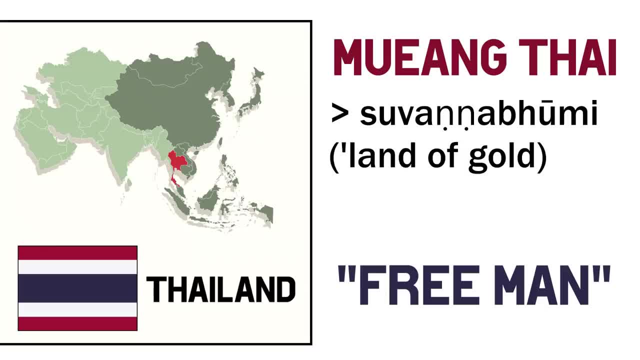 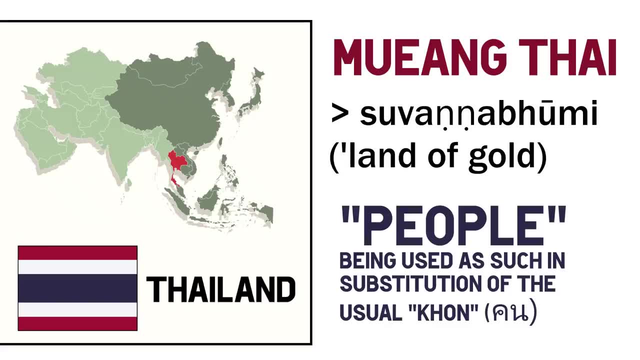 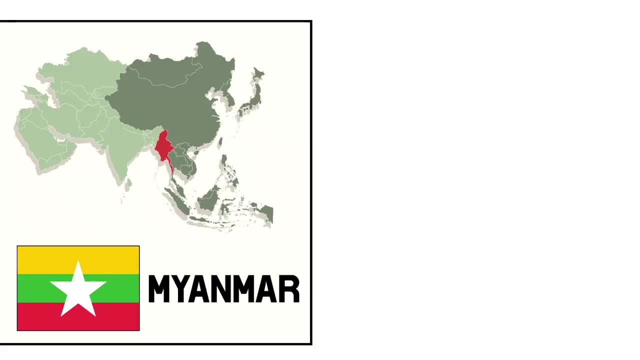 free man in the Thai language, but an actual Thai scholar argued that it simply means people or human being, since his investigation showed that in some rural areas the word Thai was used as people instead of the usual con. The second country that changed its name kind of is Myanmar, previously known as Burma. 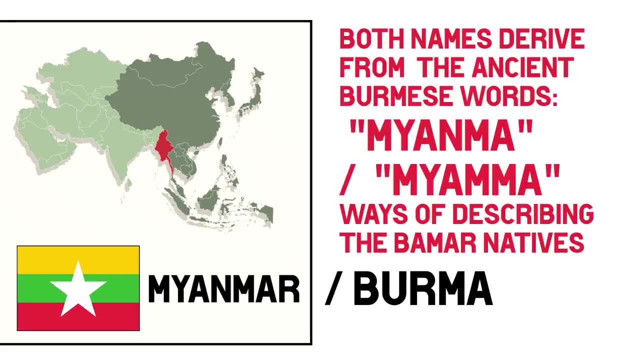 Apparently, in Burmese the origin of the two words is common and even its pronunciation is similar, and it seems that many countries either still use Burma when referring to it or use both terms, So maybe saying that it changed its name is an overstatement. Both 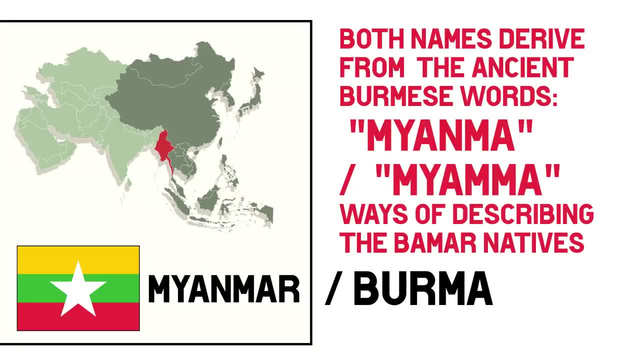 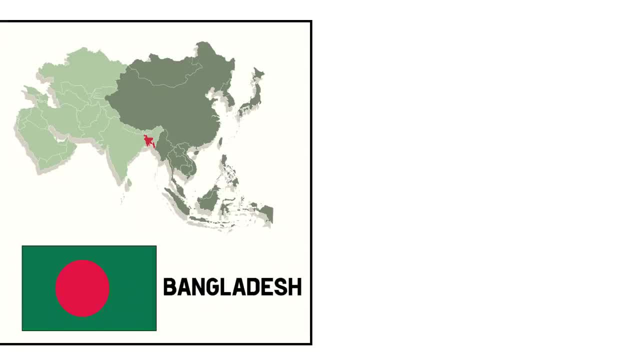 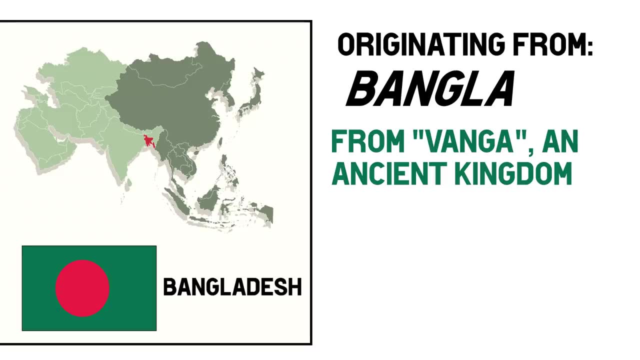 names derive from the earlier Burmese language, from the words Myanmar or Myama, a way of describing the Bamar natives which mostly inhabited the region West Bangladesh Bangla. Its exact origin is unknown, but some believed it comes from Vanga, an ancient 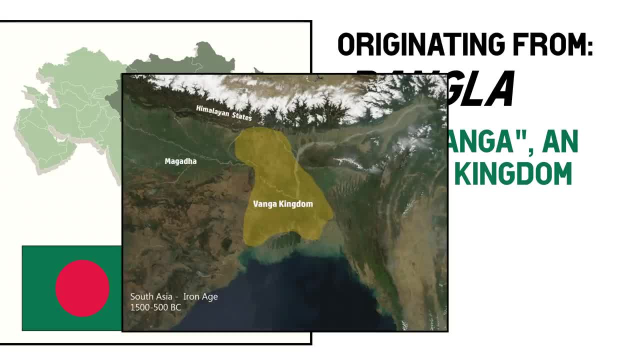 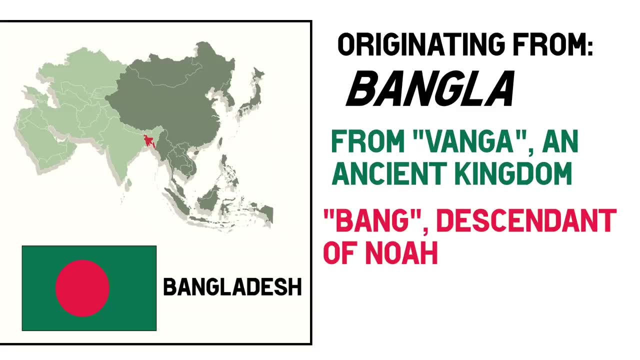 kingdom which was located on the Ganges Delta. Religiously, it is said to come from Bang, a descendant of Noah, who would have initially colonized the area. The suffix al- apparently comes from mounds of land which the ancient Rajas had raised from the ground. perhaps. 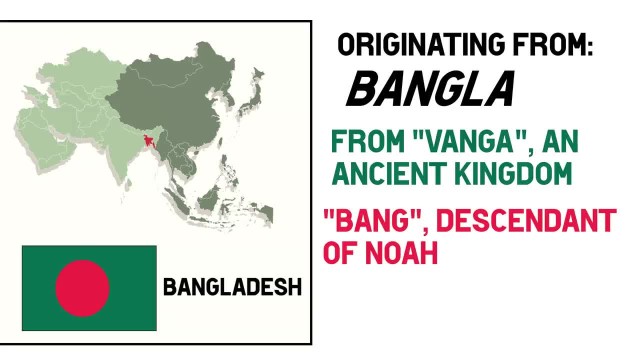 for defensive purposes. Other, more straightforward theories state it means land of the Bengal, since the general area in which Bangladesh is located is known as Sambar And, in fact, the Sultanate of Bengal from the 14th century included what is now the. 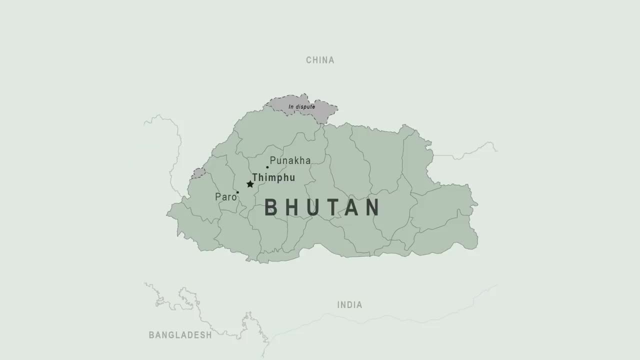 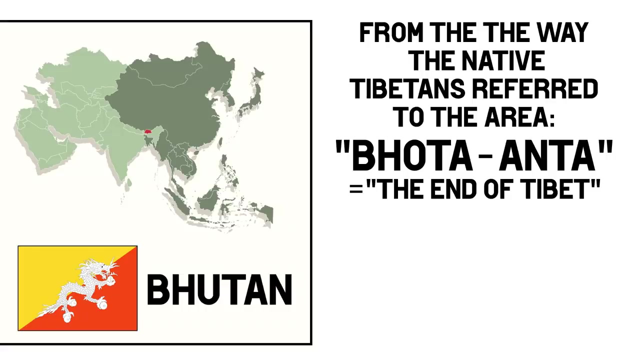 country Going north, Bhutan. The precise etymology of Bhutan is unknown, but it's likely to derive from the way the native Tibetans referred to the area Bodh, more precisely Bhota Anta in Sanskrit, meaning the end of Tibet, since Bhutan is located on the southern extremity. 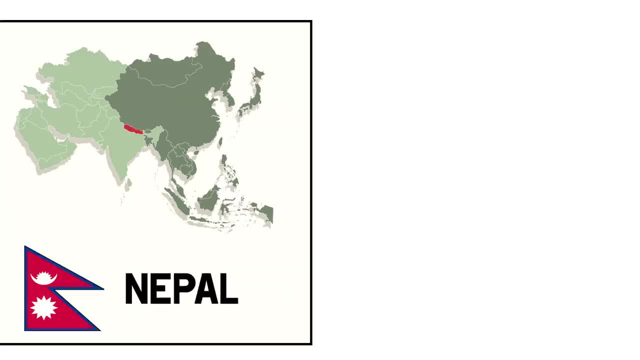 of the Tibetan Plateau And, somewhat next to it, Nepal. According to Hindu mythology, Nepal derives its name from an ancient Hindu sage called Ne. However, some people who have studied the name state that Nepala was a joining of two local words, Nipa meaning. 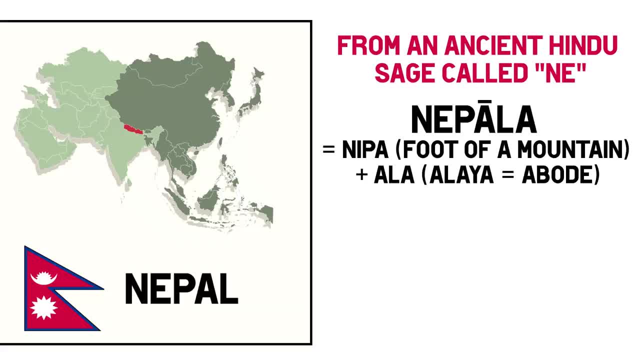 foot of a mountain and Ala short for Alaya and meaning abode, And so Nepal would mean abode at the foot of the mountain. It also has been proposed that the origin would be Nepa, from Tibeto-Burman and joining the words of Ne cattle and Pa keeper, since that. 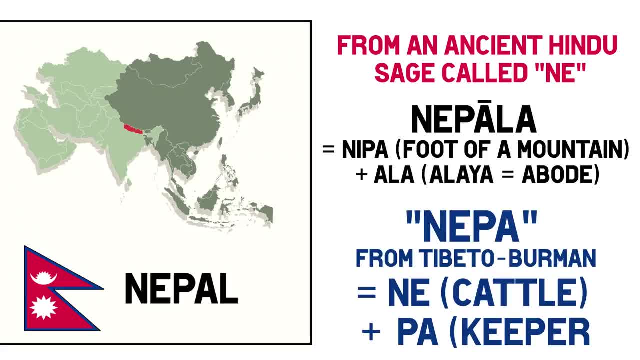 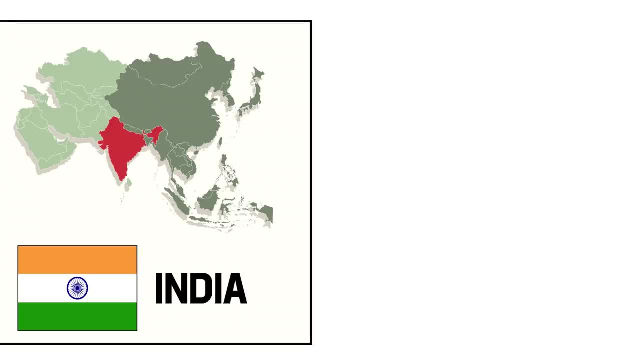 was apparently an activity of the locals. It's interesting to see how many of these country names all over the world are just of unknown origins, simply having passed down from generation to generation, Moving to one of the biggest countries in Asia. the name India is derived from the name. 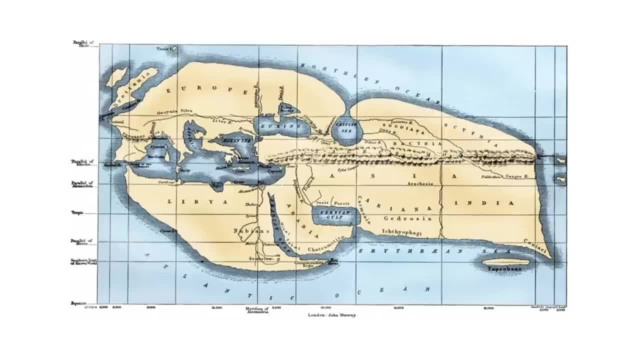 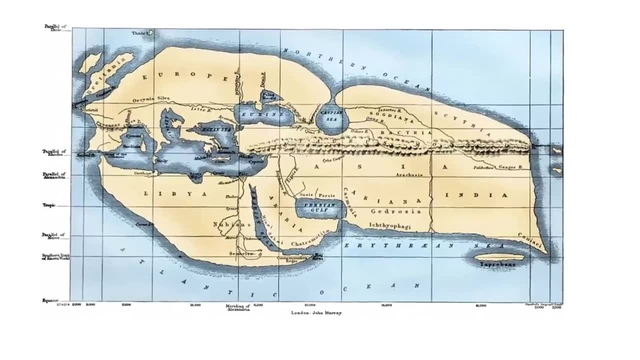 of the river Sindhu or Indus, and has been in use since Greek writer Herodotus first used it in the 4th century. It was precisely the ancient Greeks who began referring to the ancient Indians as Indoi, meaning people of the Indus river valley. 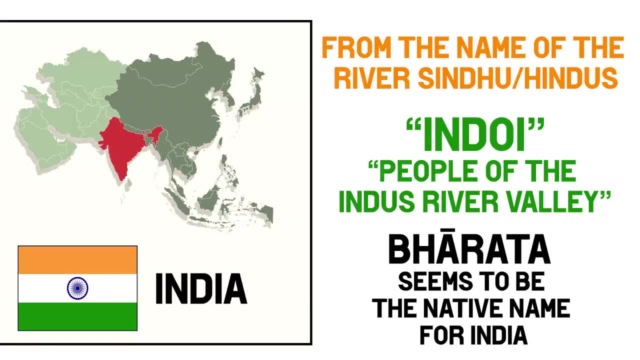 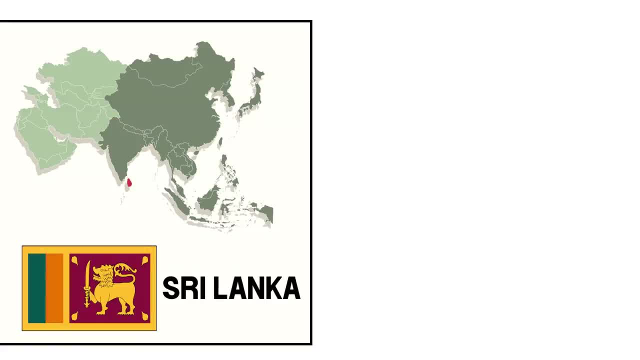 Bharata seems to be the native word for India, and please correct me if I'm wrong, but it is said to be derived from the name of an important religious figure And a smaller island south of it, Sri Lanka. Sri Lanka has had many names throughout history. 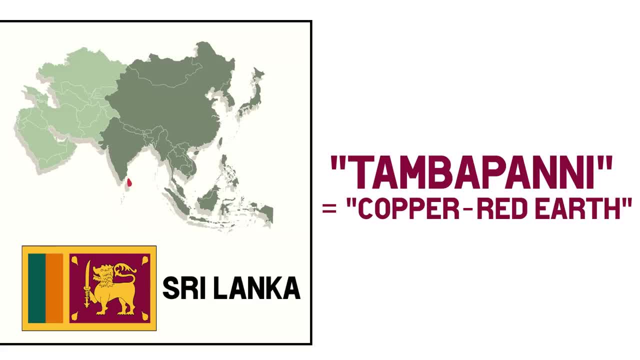 as well from Tambapani, meaning copper red earth. Ancient Greek geographers called it Taprobana. the Portuguese named it Ceylon, which the English then translated to Ceylon. The origin of Ceylon seems to be the Latin Ceylon, which the Romans would have named. 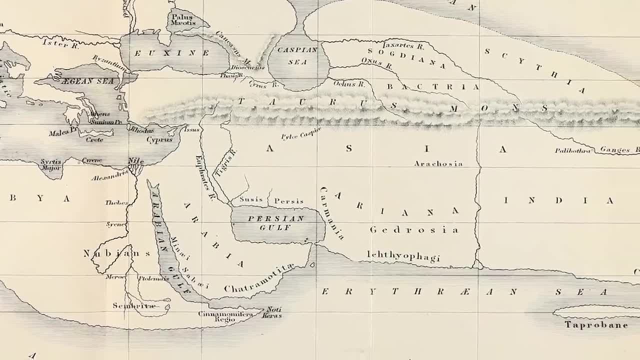 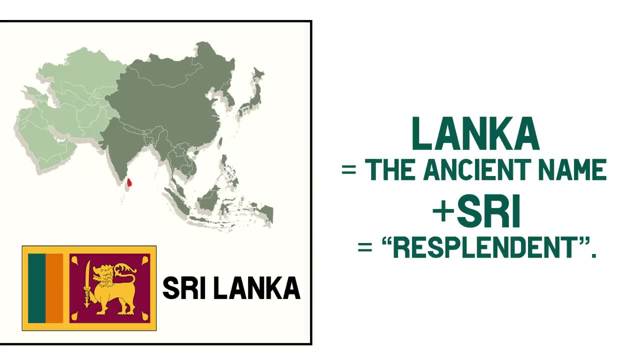 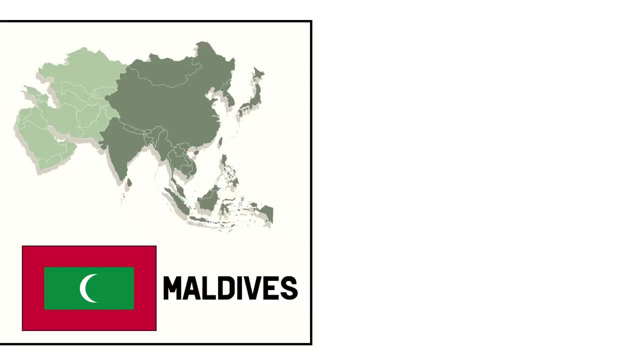 it. But did the Romans even know about Sri Lanka? I thought they hadn't established communications with people that far away. The current name of Sri Lanka divides itself into Lanka, the ancient name of the island, and the ancient name of the island. The name of the island is also known as the Maldives. 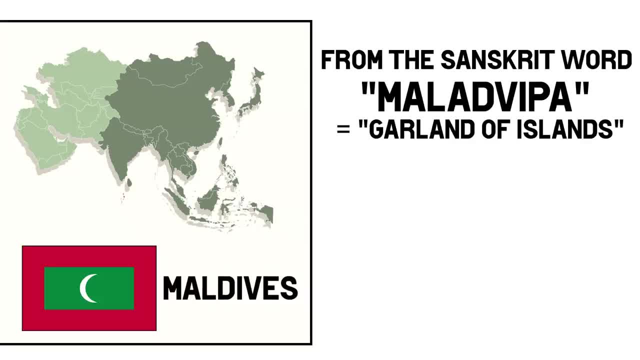 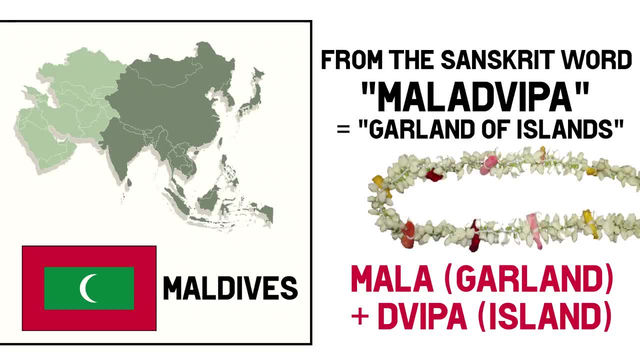 which probably get their name from the Sanskrit word Maladvipa, meaning garland of islands, From mala, garland and vipa, an island. Garland means a wreath of flowers. I had to go look it up. Back to the mainland, we have Pakistan. The name of the country was coined in 1933 as 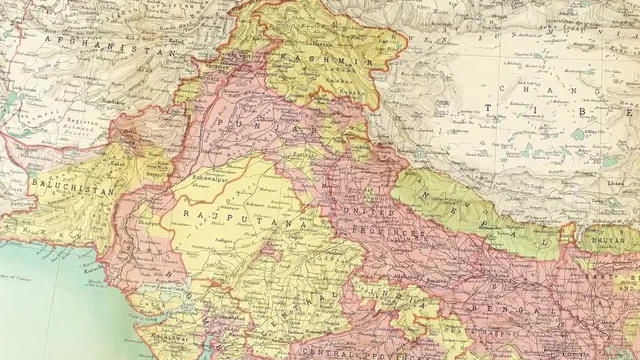 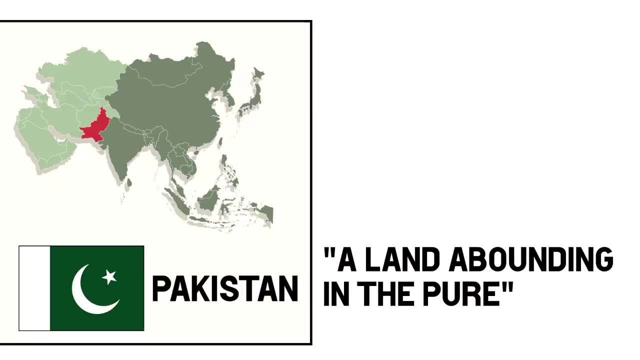 an acronym referring to the names of the five northern regions of the British Raj: Punjab, Afgania, Kashmir, Sindh and Balochistan. If translated literally, it means something like a land abounding in the pure, in reference to the word Pak, meaning pure in Persian and Pashto, and the suffix Istan, which means 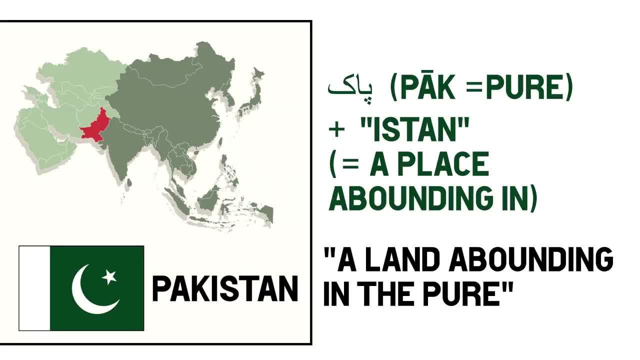 a place abounding in so like place of X. This is why so many of the country names in these areas end with Istan. And now, precisely to the Central Asia Istans, starting with Tajikistan. Tajikistan means land of the Tajiks. Tajik is most likely the name of a local tribe which 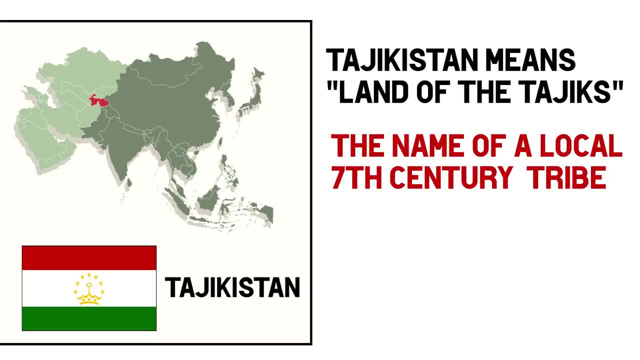 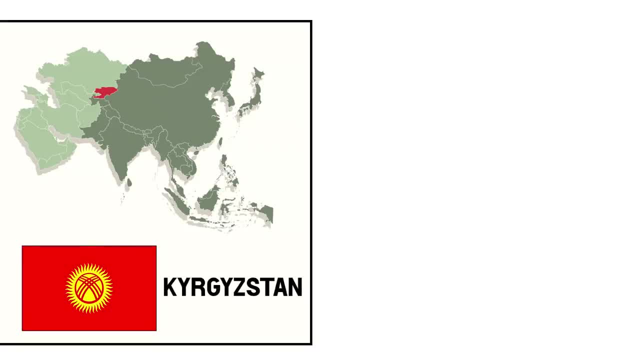 lived there in the 7th century. The title Tajik also served to differentiate these people from the abundant Turks or Mongols that lived in the region Then Kyrgyzstan. Kyrgyzstan is believed to come from the Turkish word for 40, referring 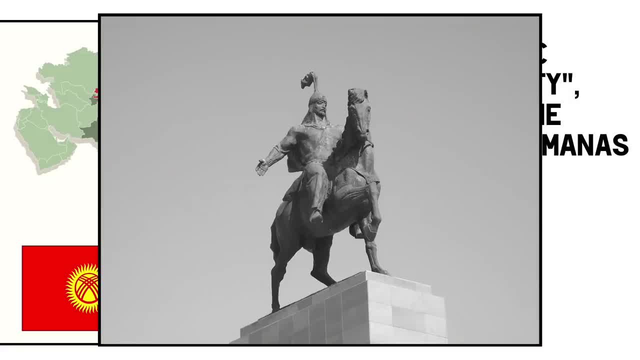 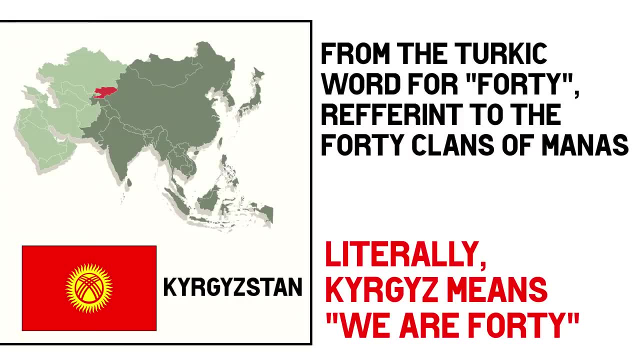 to the 40 clans of Manas. Manas is a legendary local hero who supposedly united 40 regional clans against an external invader, And literally Kyrgyz means we are 40. Kazakhstan- Kazakh also has a Turkish origin and means to wander, reflecting the Kazakhs'. 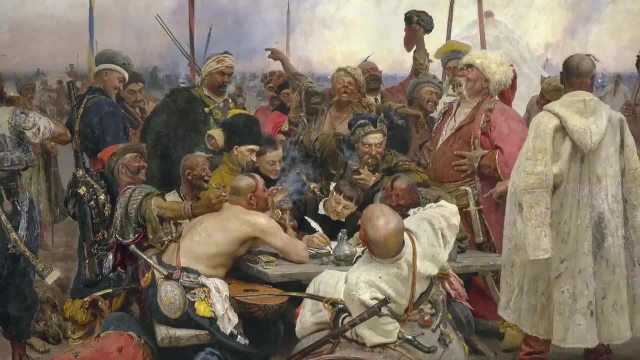 nomadic culture. The name of the region is Kyrgyzstan. The word Kyrgyz stands for the Kyrgyz people. The term Cossack, often well known for the role of the Cossacks in Russian history, especially military-wise, has the same origin. 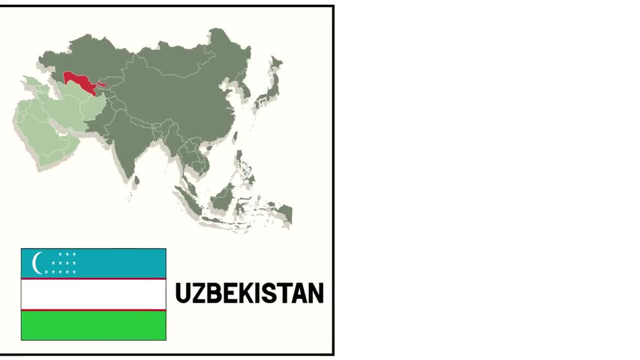 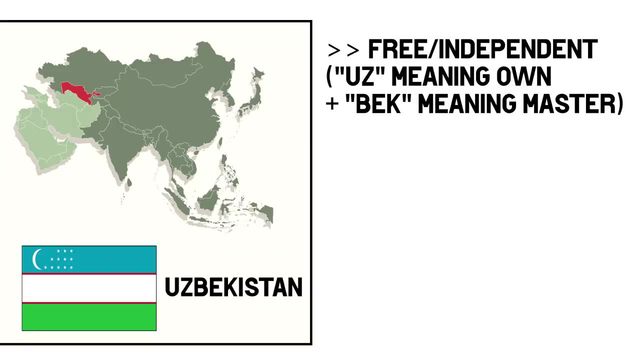 Uzbekistan has the common Istan suffix, meaning land of something, but this something has three options. Apparently, the exact origin is unknown. It either means free, slash, independent, joining the Turkish words uz, meaning own, and bek meaning master, being your own master. 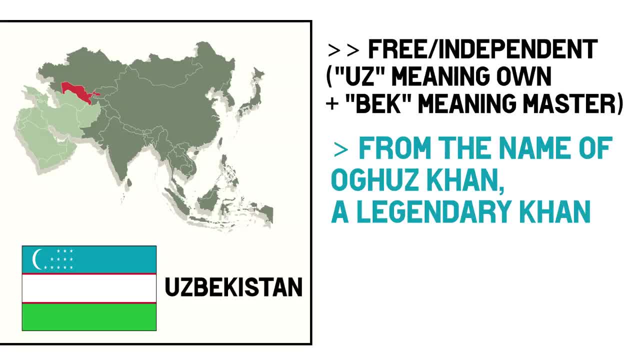 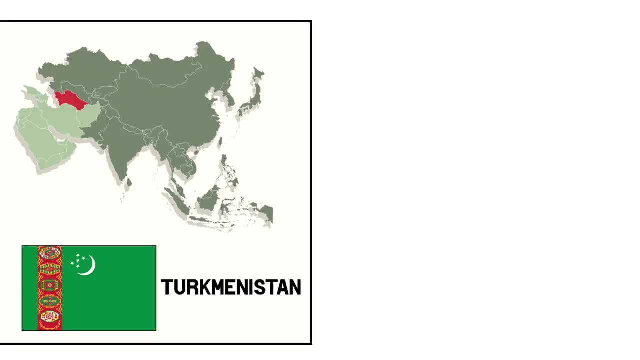 or it comes from the name of Oguz Khan, a legendary khan of the Turkish people, or from the local Oguz tribe And Turkmenistan, which has two possible origins that are completely opposite to each other. It could either come from Turk plus the suffix men, meaning almost Turk in reference to 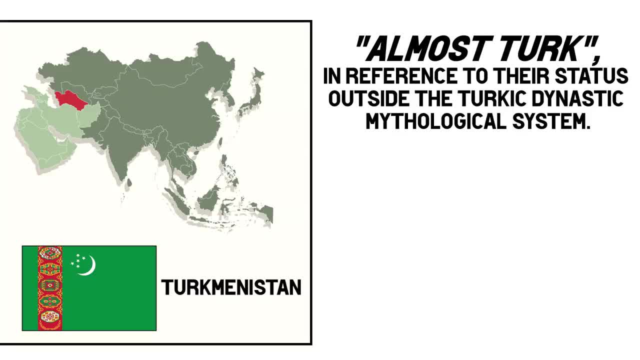 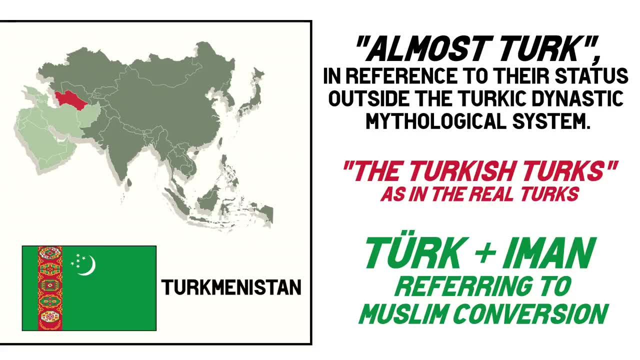 their status outside the Turkish dynastic mythological system, or it could mean the Turkish Turks, as in the real Turks. Some religious chroniclers have also suggested that it came from the word Turk and iman, in reference to a massive conversion to Islam. 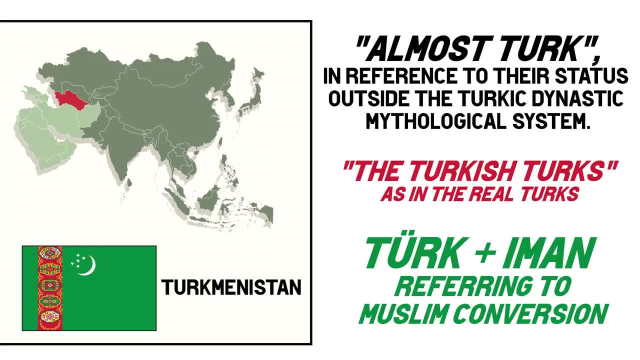 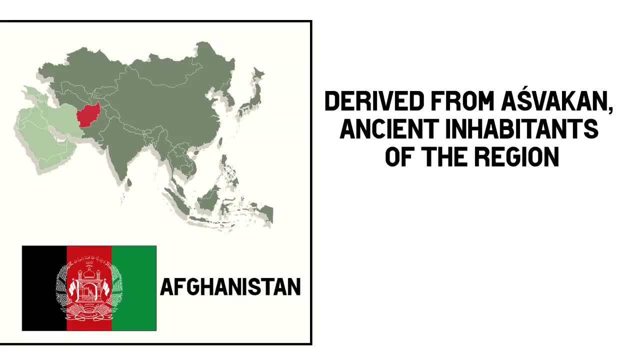 of the territory in the 10th century, Also in Istan, but not usually associated with that group of ones. we just saw Afghanistan. The root name Afghan is, according to some, derived from the name of the Azvakan ancient inhabitants of the region, while Azvakan literally. 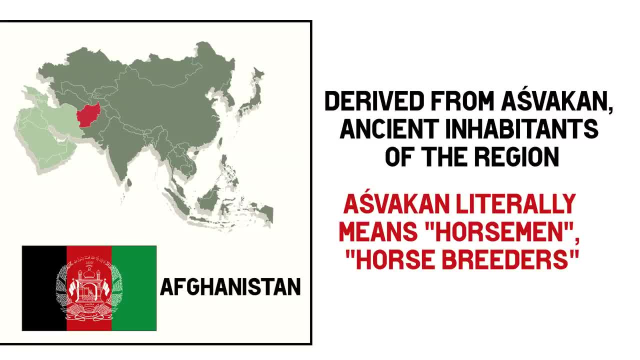 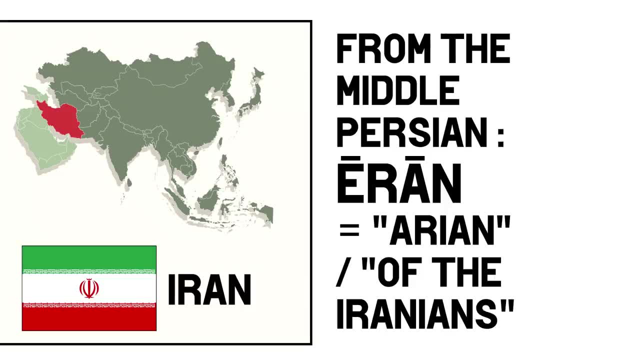 means horsemen or horse breeders, so cavalrymen. Closing in on the Middle East, Iran, It derives directly from Middle Persian Edan, meaning Aryan, and so it's sort of land of the Iranians. As far as I could understand, Iran has always been Iran to the native population, but historically 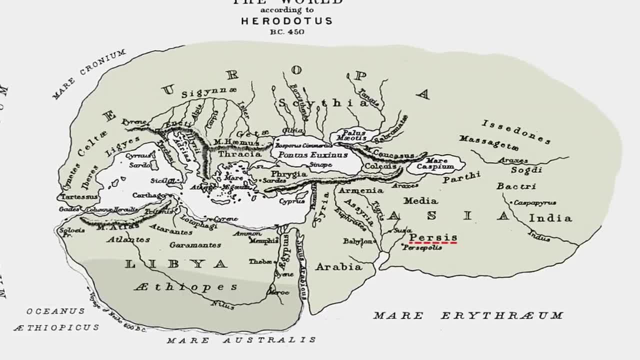 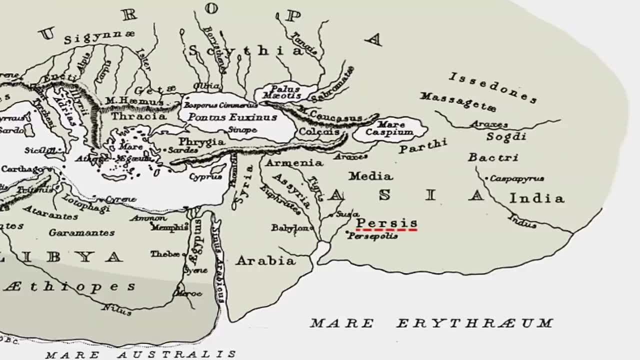 it was referred to as Persia by the West, Apparently, due to the fact that Iran is a land of the Persians, it was also referred to as Persia by the West In 1935, they requested that the international community should refer to the country by its native name, Iran, And 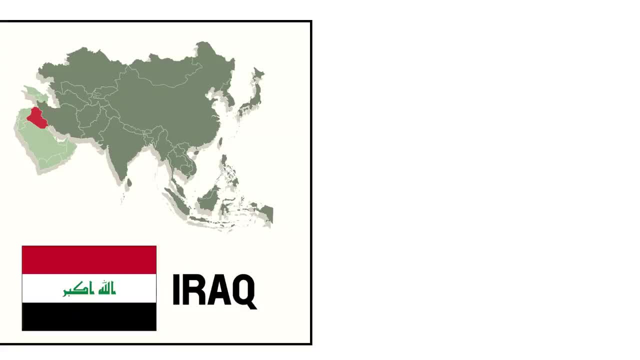 with a very similar name but with a different origin: Iraq. Iraq probably has one of the oldest continuous names. The Arabic version has been in use since at least the 6th century. There are several suggested origins for the name. One dates to the ancient Sumerian city. 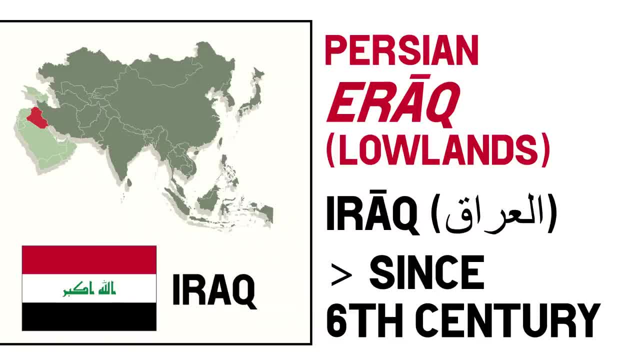 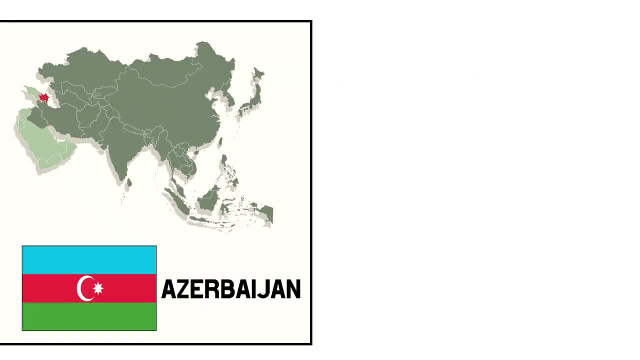 of Uruk. Another is from the Middle Persian word Iraq, meaning lowlands, And the traditional meaning associated with it means well watered and fertile. Onto the Caucasus region we have Azerbaijan, which seems to get its name from a nobleman. 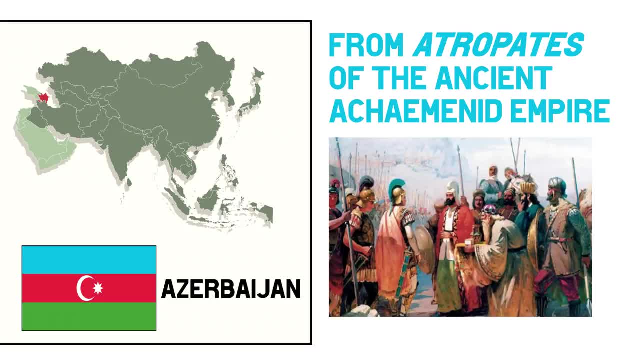 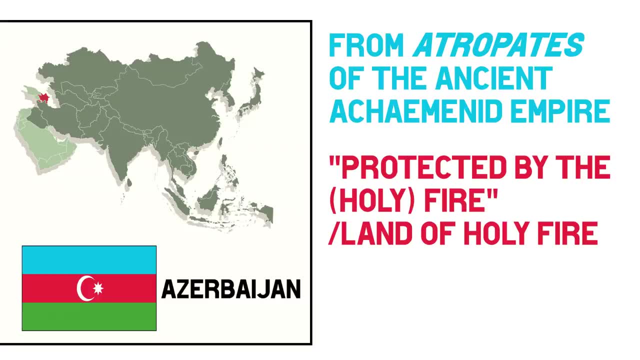 of the ancient Achaemenid Empire called Atropats. The name Atropats itself is the Greek translation of an old Iranian name with the meaning protected by the holy fire. There are also some theories that the name would derive from the Zoroastrianism religion. 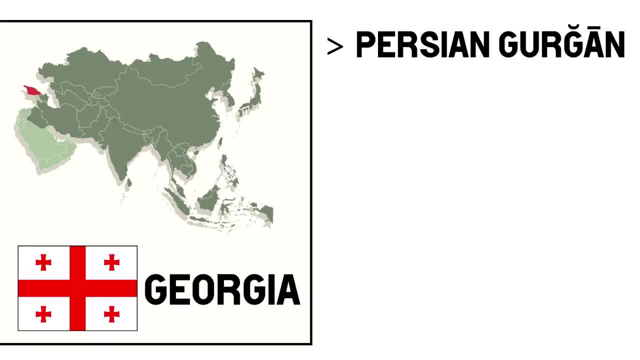 Then Georgia, which probably stems from the Persian designation of the people who inhabited the ancient Persian region, Gorgan. this term itself might have been established through the ancient Iranian designation of the land by the Caspian Sea, which was referred to as Gorgan, land of the wolves, But it could also just be a translation of the saint which: 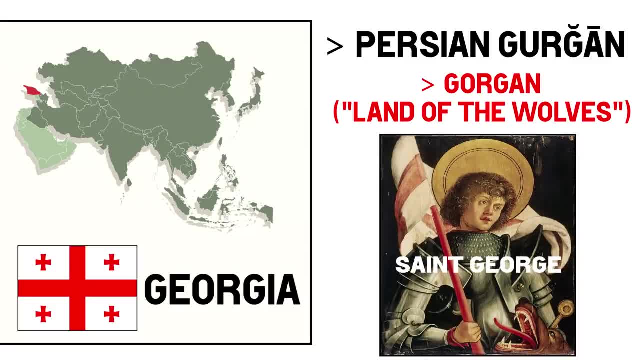 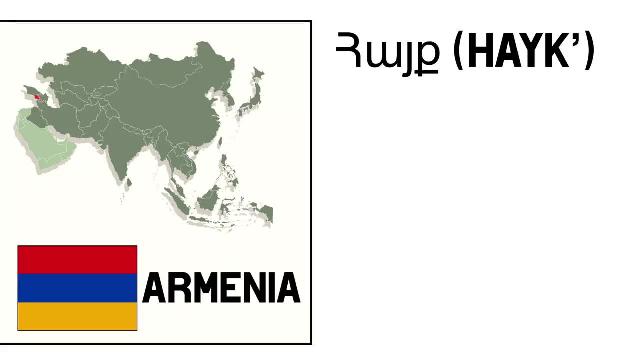 was apparently extremely popular among the local population: Saint George, And also Armenia. The original native Armenian name for the country was Ayk, with the Persians even calling it Ayastan at one point, And this Ayk name would come from Ayk himself. 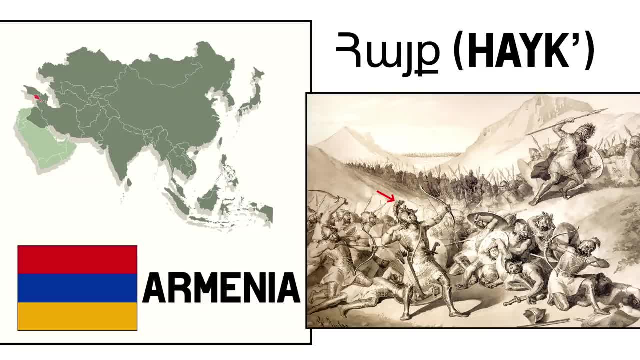 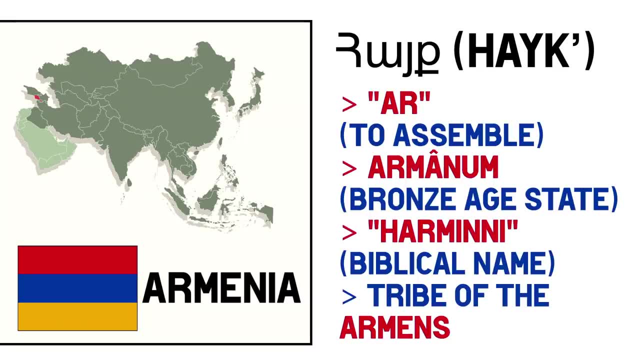 the legendary patriarch of the Armenians and great, great, great, great, great, great great grandson of Noah. When it comes to the modern Armenia itself, the origin is uncertain and has many options, The Indo-European R meaning to assemble the Bronze Age state of Armanum. 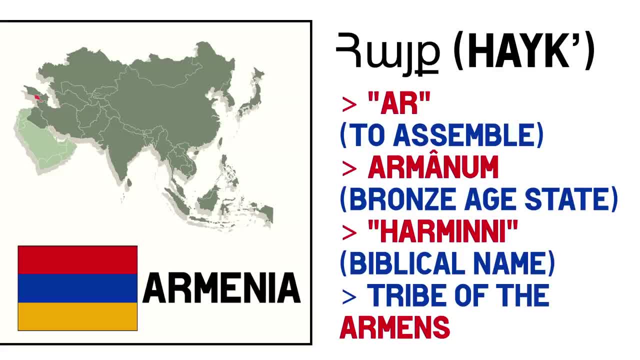 from Armini, meaning the mountainous region of the Minni, which is apparently a biblical name for the region, and some even speculate there was a Bronze Age tribe called the Armens, who would have originated the name Onto the Mediterranean coast, Syria. Syria's name seems to come from the ancient name of 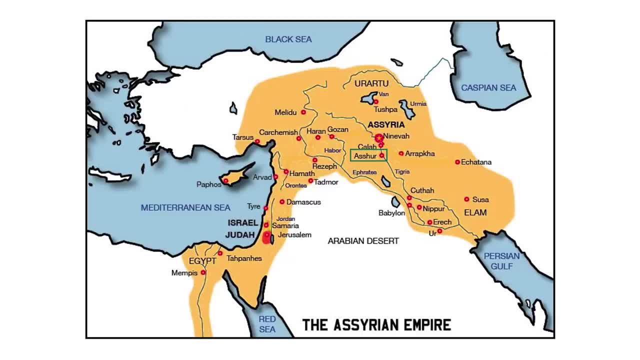 Assyria in northern Russia. The name Assyria comes from the ancient name of Assyria in southern Mesopotamia, which in turn derives from the ancient Akkadian word Asshut, precisely the capital of the ancient Assyrian empire. I couldn't find the official origin for 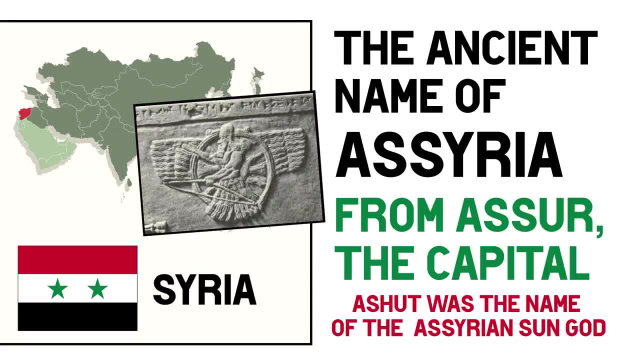 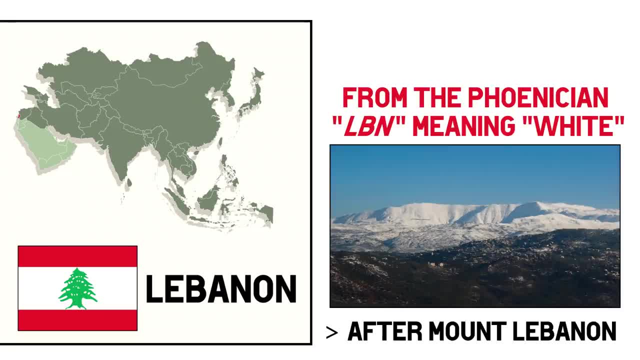 this, but it seems Asshut was the name of an Assyrian god representing the sun, so maybe that could be the origin, Then Lebanon, which seems to be named after Mount Lebanon, located in the country. The name of the mountain comes from the Phoenician. 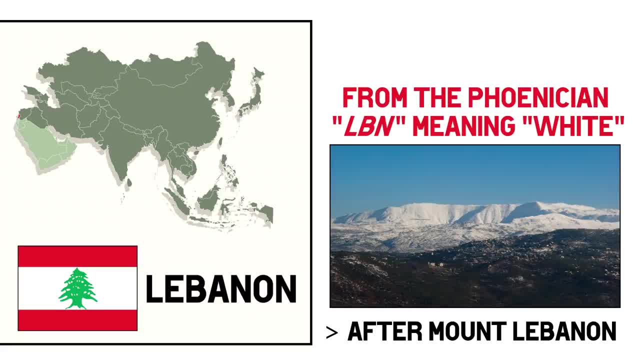 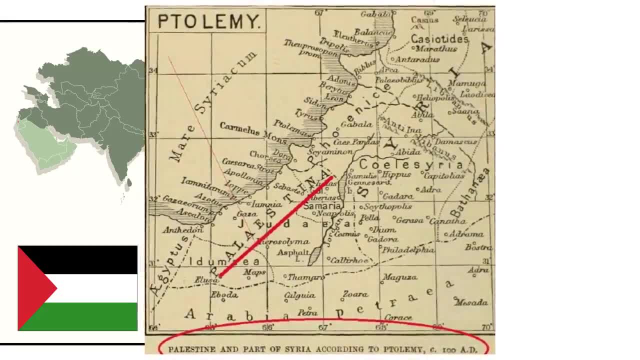 root Eben, meaning white, in reference to the snow at the top of it. Moving to Palestine, it has been used as a term for a very long time to refer to the general region in which the state is located. Historically, it seems to date back at least. to the times of ancient Greece, with Herodotus being the first historian to write, in the 5th century BC, about a district of Syria called Palestine. The term itself in Latin Palestina is thought to have been coined precisely by the ancient Greeks to describe the area occupied. 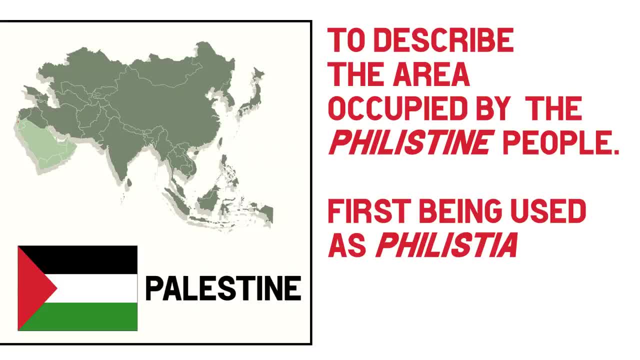 by the Philistine people, first being used as Philistia and then evolving to Palestine, Although some say it might come from a native word, peleshet, which would roughly translate to migratory, also referring to the Philistine people And then Israel. under the British mandate, the whole region was known as Palestine. When, 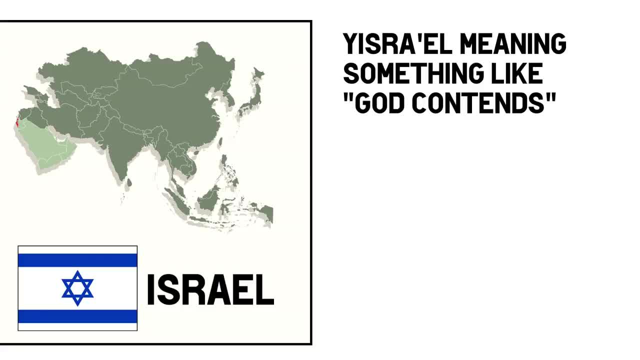 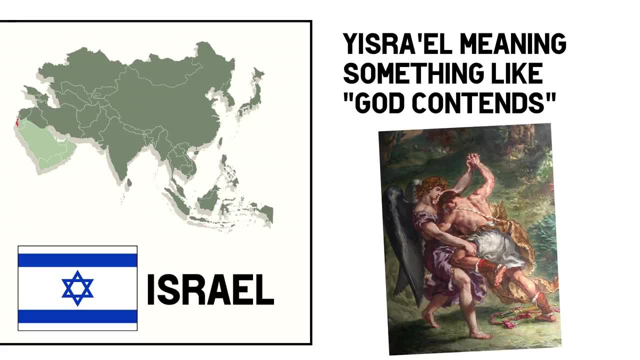 Israel became a state. it chose this name From the Hebrew name Yisrael, meaning something like God. contends In the Old Testament, Israel, who was formerly named Jacob, wrestles with an angel. apparently, To the west is Jordan which takes its name. 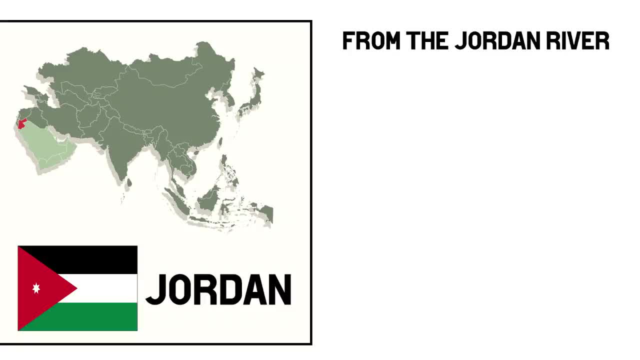 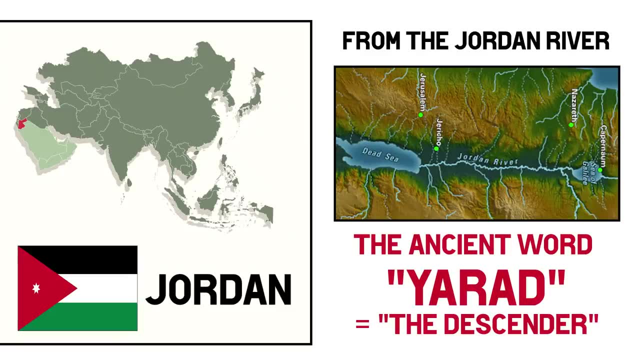 from the Jordan River, which forms much of the country's northwestern border. The origin of the river name itself seems to be the ancient word Yisrael Yarat, meaning the descender, reflecting the river's path And on to another big country, Saudi Arabia, With the joining of the kingdoms of Ejaz and 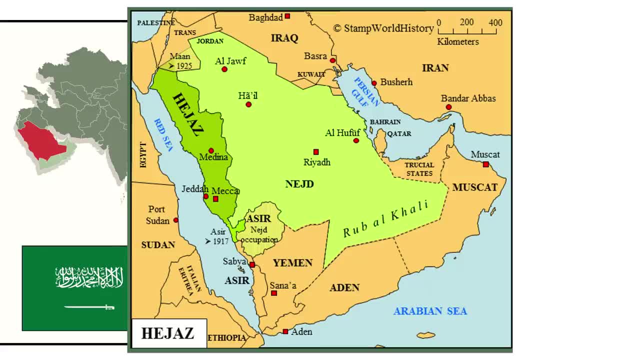 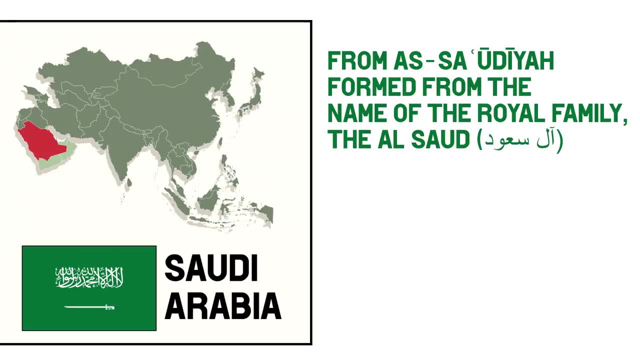 Naid, it was named the Saudi Arab Kingdom. Usually it is commonly known as Saudi Arabia. The word Saudi is derived from the element As-Saudiyah in the Arabic name of the country, formed from the dynastic name of the Saudi royal family, the Al Saud. Its inclusion expresses: 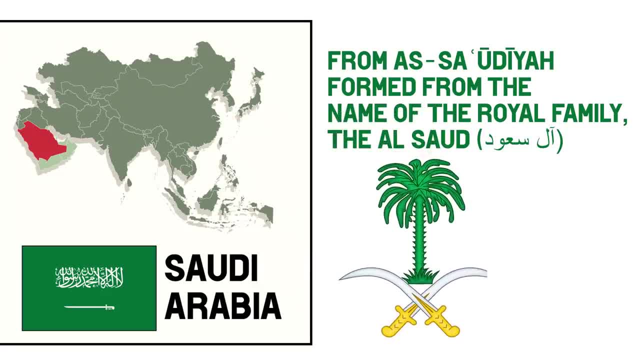 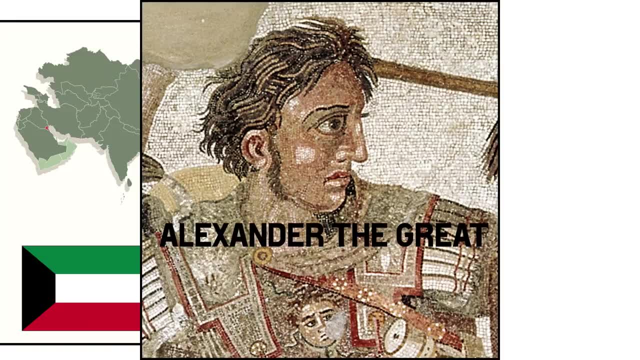 the view that the country, an absolute monarchy, is under the possession and control of the royal family. Moving to the small nation of Saudi Arabia, Saudi Arabia is known as the Kingdom of the Arab Emirates. In the 4th century, the Bay of Kuwait was colonized by Alexander the Great and the Greeks. 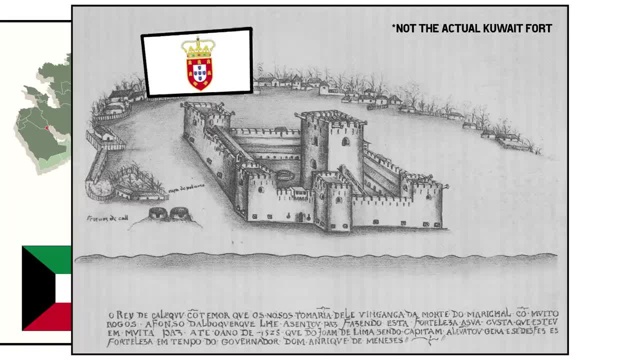 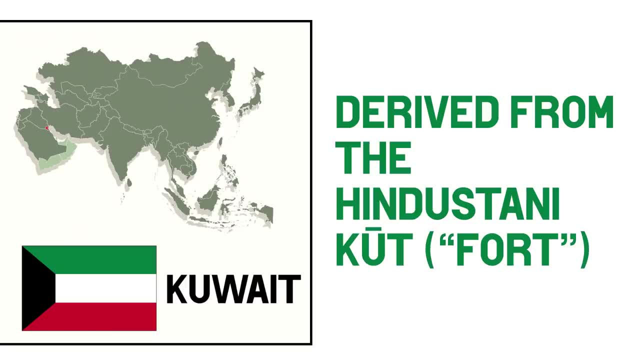 named it Larissa. Eventually it became a colonial fortress of the Portuguese in 1521.. The Hindustani word for fort was Kut, and so that would eventually become Kuwait, Joining seven emirates, the United Arab Emirates. The most well-known are Abu Dhabi and Dubai. 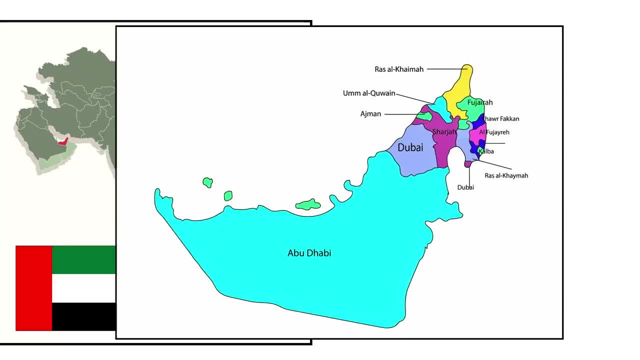 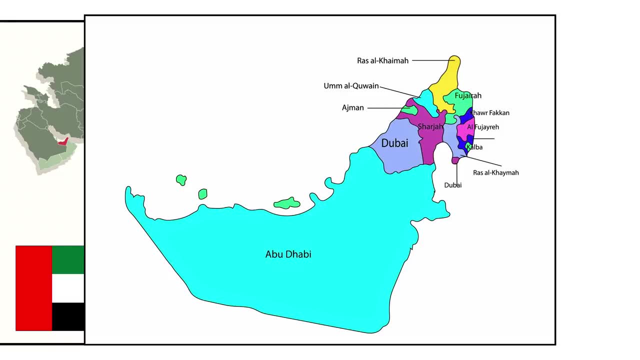 but there are five others: Ajman, Fujairah, Raz al-Kaimah, Sharjah and Umm al-Qawain. UAE means precisely that It's a union of eight. Abu Dhabi is the name of Arab Emirates. An emirate is a political territory ruled by. 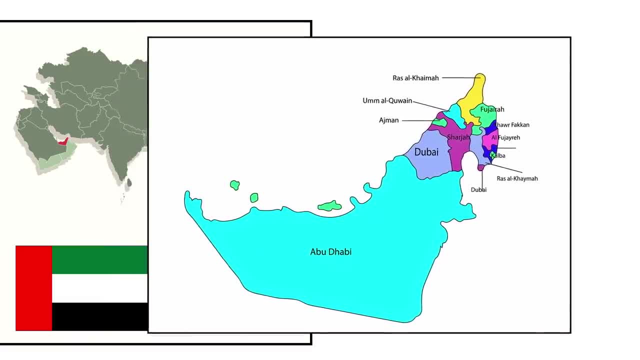 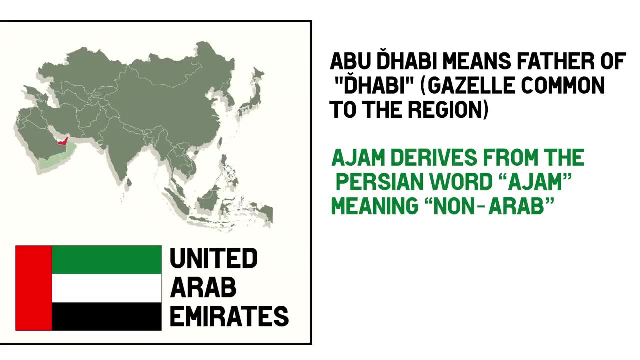 a dynastic monarch, an emir. But what about the names of these individual emirates? Abu Dhabi means father of Dabi, a type of gazelle common to the region. Ajman is named after its capital city, which apparently derives from the Persian word Aja, meaning non-Arab. Dubai might come from the word Daba. 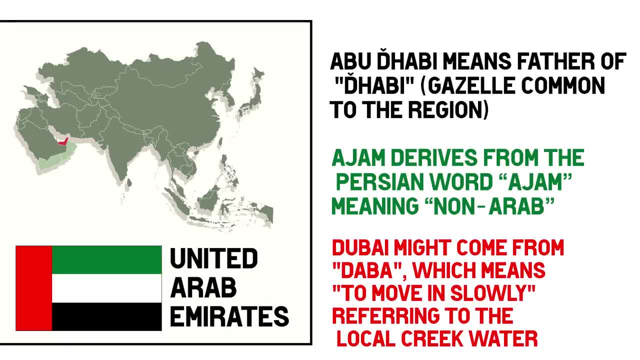 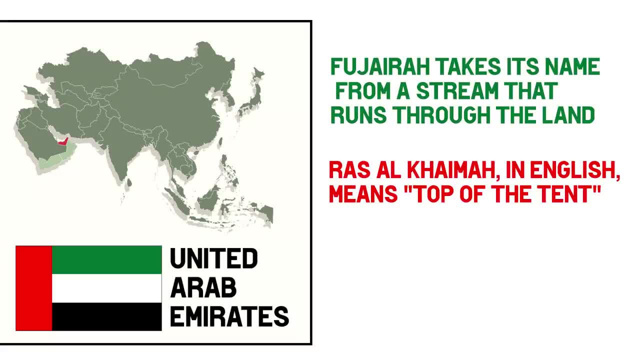 which means to move in slowly, referring to the slow waters of the Dubai creek. but there are also other options. Fujairah takes its name from a stream that runs through the land. Raz al-Kaimah in English means top of the tent. Sharjah might come from the name of an. 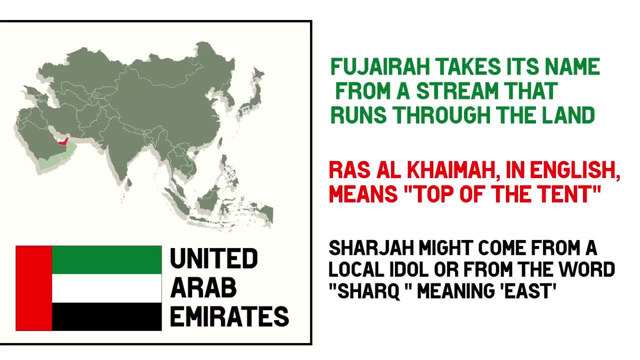 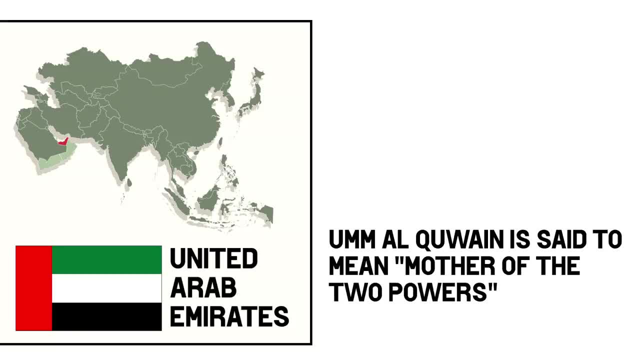 idol worshipped in the ancient era, or from its location east of Dubai, And Umm al-Qawain is said to mean mother of the two powers Not part of the UAE but pretty much adjacent to them- Qatar. A Roman writer called Pliny the Elder wrote in the first: 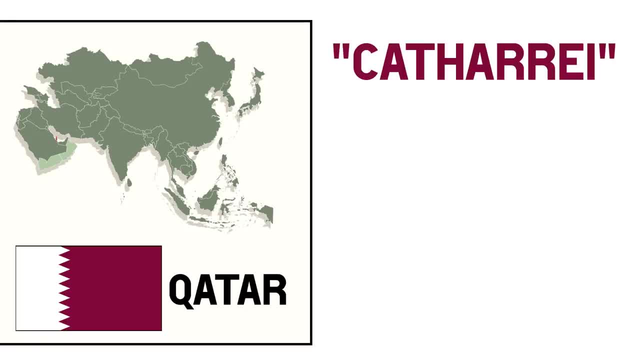 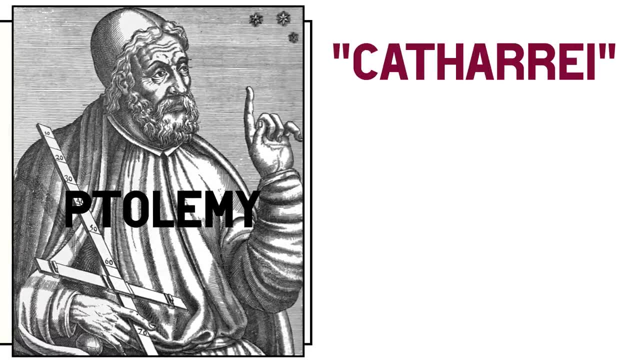 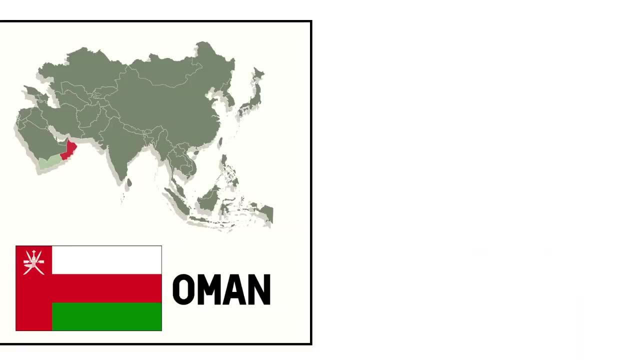 century about the inhabitants of this peninsula, and he referred to them as Qataghay, likely coming from the name of a local settlement. A century later, Ptolemy drew the first known map of the region, Next Oman, With an uncertain origin. the most likely hypothesis is that the name comes 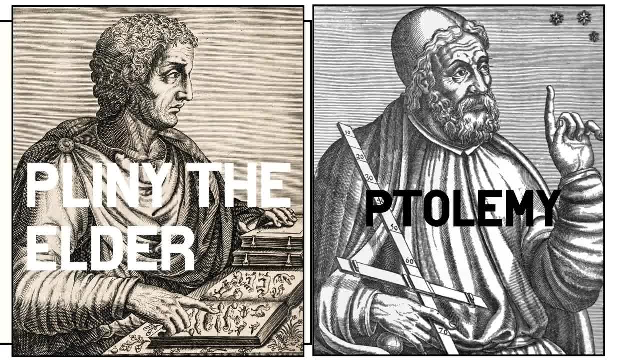 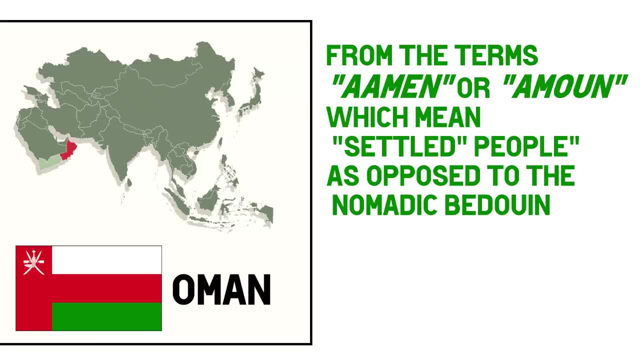 from the way Pliny the Elder and Ptolemy described the region in ancient times: Omana and Omanon respectively. In Arabic, the name of the region is typically seen as coming from the terms Aman or Amun, which means settled people as opposed to the nomadic Bedouin Others.